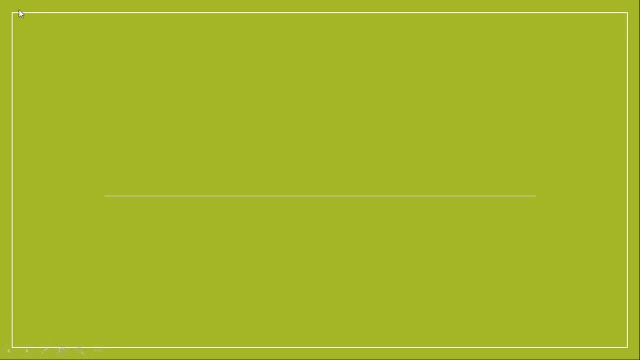 So hello and greetings to all the viewers. Today we will going to see introduction to practical finite element analysis. So in this video we will go through the complete overview of what is FEA. So, from basics of FEA, from solution of engineering problem to the. what are the elements which will come under FEA, like elements, nodes, stiffness matrix, how to form stiffness matrix, then different types of elements. 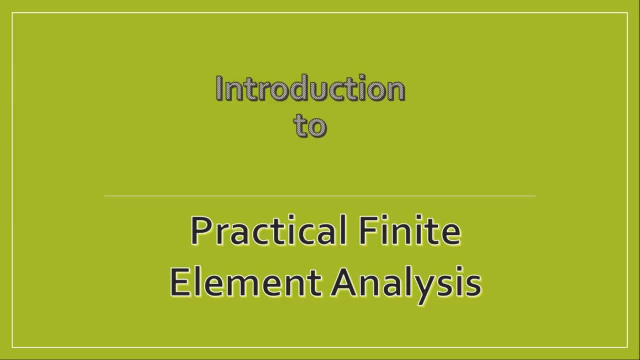 Different types of analysis, different types of softwares available for CAD as well as for CAE, whether they are paid or free softwares. Then we will discuss different types of analysis and then we will go through some of the examples of practical FEA. So keep watching this complete video up to end so that you will get the complete overview of practical finite element analysis. 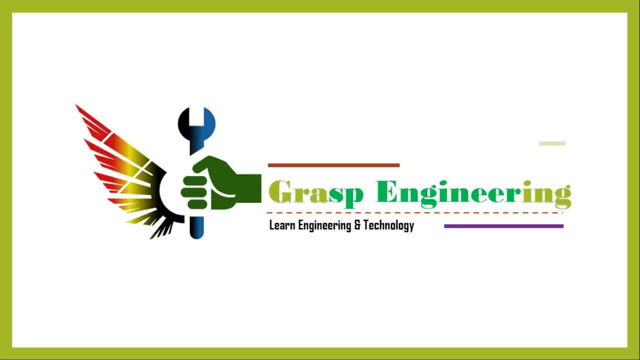 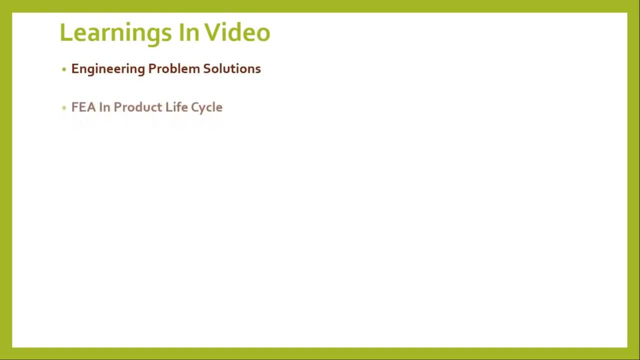 So now this slide will present the learnings in this video. First we will see the engineering problem solutions, then FEA and product life cycles, Then we will go through the different numerical methods. Then we will discuss about what is FEA and FEM. Then we will go through the discretization of a problem, Then degrees of freedoms, nodes, elements, types of elements, meshing, accuracy. 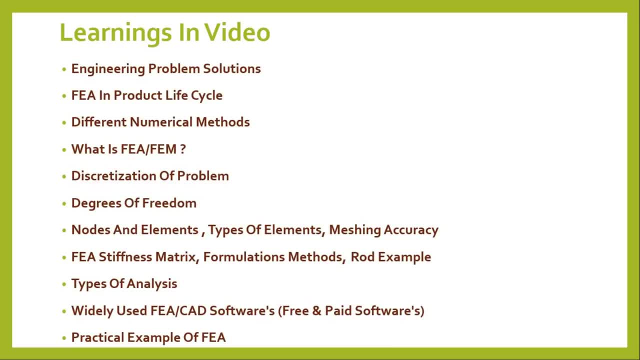 the FA steepness matrix formulation methods and one of the example like rod bar element example. then we will go through the what are the different types of analysis and then we will discuss widely used FA CAD software like free and paid versions. then we will discuss 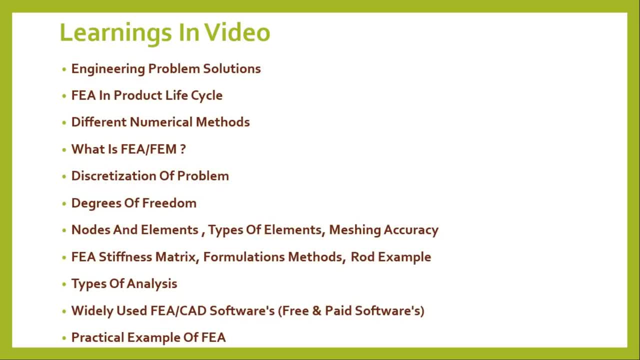 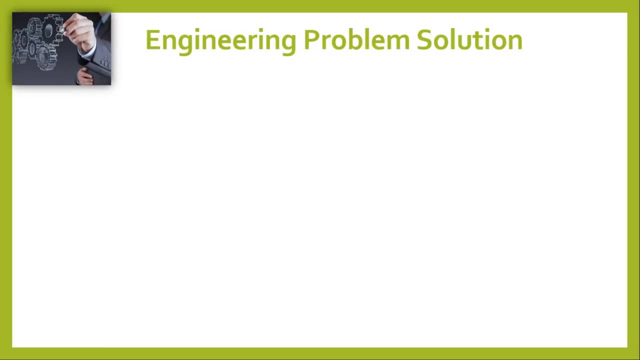 the practical examples of finite element analysis. so once you will go through this old terminology you will get some of the overview of practical finite element analysis. the first we will discuss about the engineering problem solutions. so there are like three basic methods to solve any engineering problem. the first is nothing but your analytical method. 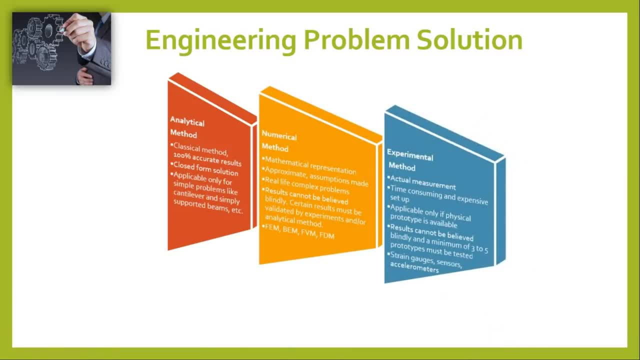 and the another is like your numerical method, and then the next is nothing but your experimental method. when we talk about analytical method, it is like hundred percent accurate classical method, which is closer from the solutions and applicable for a simple problem like cantilever beam and simply supported beam. you can take example of G-PREM. this here is like a cantilever beam. 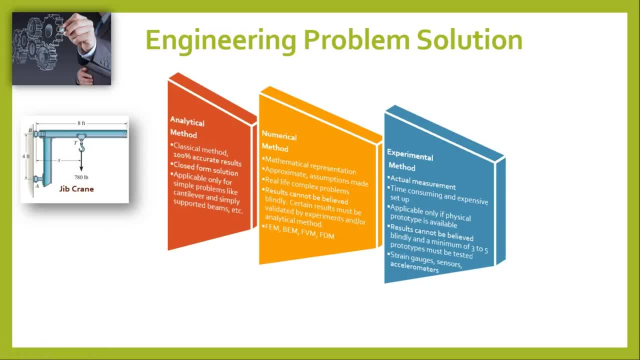 when the problems are simplified, or you can say the simple problems are there, then we can easily find out the output of that problem by using analytical method. when we talk about a complex geometry, like if you consider this kind of complex geometry, like complex claim structure or any other complex, like complex geometry, like if you consider this kind of- 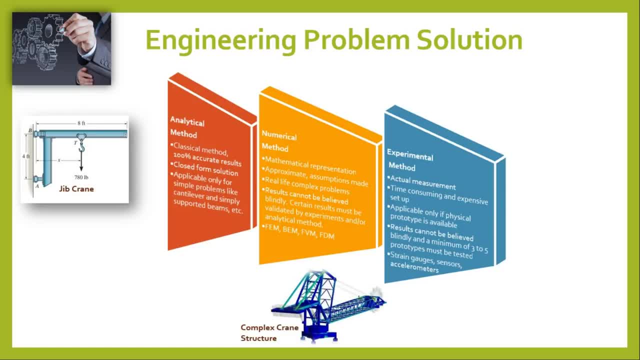 complex geometry, like complex grain structure or any other complex like complex geometry, compressor blowers. so in that case it is difficult to find out the solution by using analytical method. so in then we need this another method that is called numerical method, which is like mathematical representation, approximate assumptions based method. then real life complex problems are. 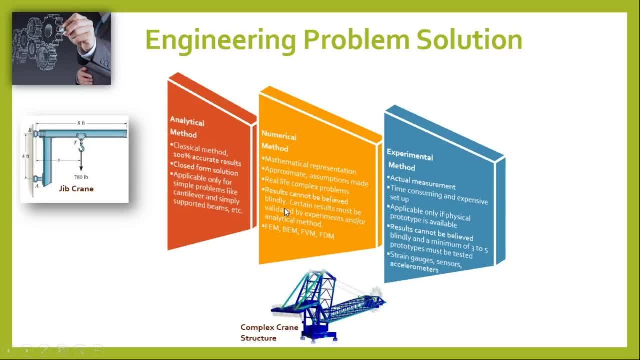 there and the results cannot be believed blindly. there is some sort of validation will be needed through by experiment or by analytical method. so under this there are like four methods: FEM- finite element method, BEM- boundary limit method, FEM- finite volume method and FDM. that is. 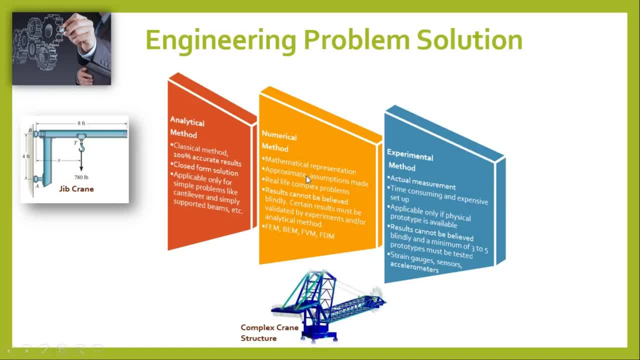 finite difference method. so most of the problems are solved by these methods. that is called numerical method. then third will come, like engineering experimental method when we try to solve. there are few examples of engineering problem solution by using experimental method. when we talk about strain gauges, sensors and accelerometers, that will give 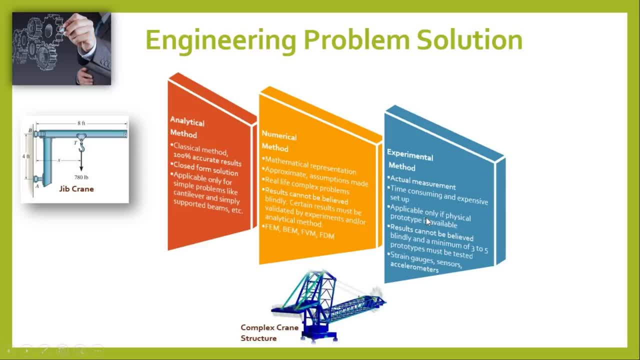 us the actual working of the equipment. so this experimental method is nothing but your actual. belongs to actual measurement. time consuming as well as expensive. setups are there and applicable only in physical prototype is available. so results cannot be believed blindly. for that we at least need a three to five prototypes must be tested. so if you take the example of this, thermal cameras. 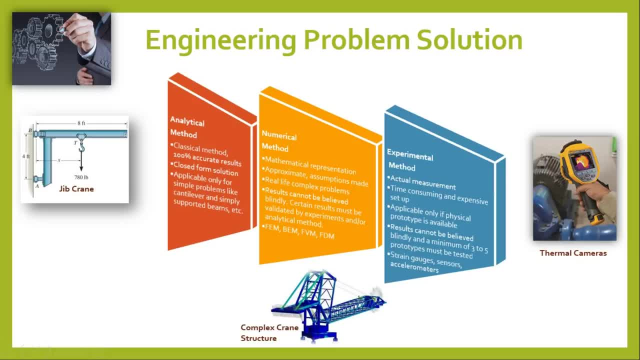 which will be detecting the temperature of this. so, like that, you can find out the solution, or you can see the temperature gradient by using this thermal cameras, or you can find out the displacement by using strain gauges, or you can find out the acceleration by using accelerometers. so they are like three major methods, like 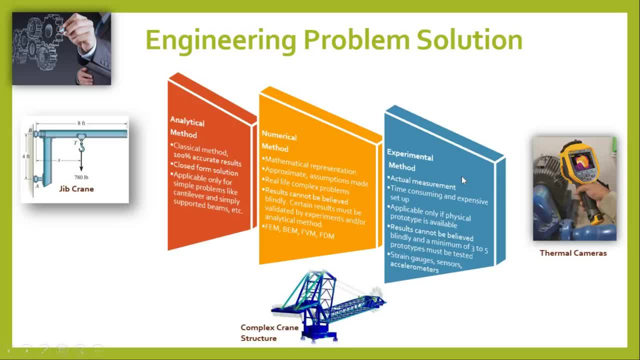 analytical, numerical and experimental to solve any engineering problems. but most of the methods lie or most of the real life complex problem will be done by using numerical method. we will discuss these methods in the next video, later sites. so as we saw about the second, that is, the numerical method is most widely used to get the engineering problem solution. so they are like four further methods are come like. first we'll talk about a few. so finite element method is a popular numerical technique used to determine the approximated solution for a partial depression equation. the applications are like linear, nonlinear buckling, thermal dynamics, fatigue analysis. the another method will come in the next video. 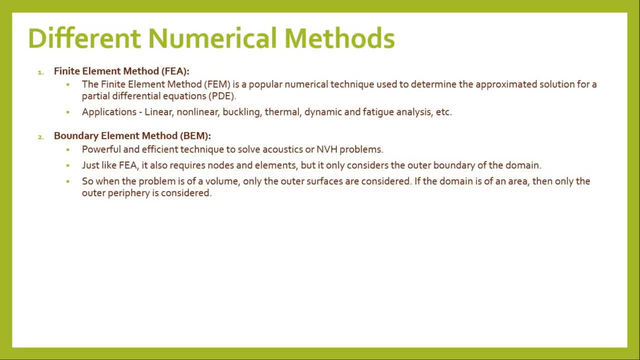 So let's have fun with it, Let's try to see what we can do with it. So you have to have your boundary element method. So in this, like a is most powerful, efficient technique to solve the acoustic as well as an RH problem, just like Fe a. 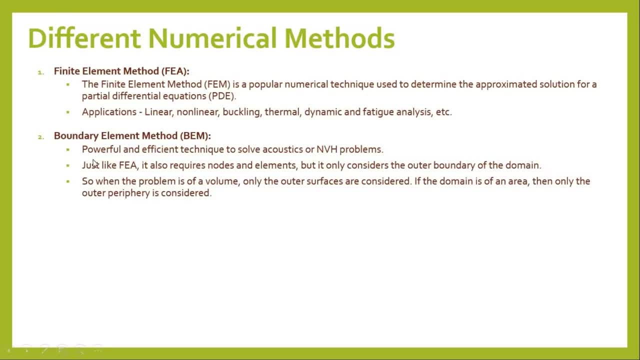 Its also pass the notes and elements, but it only considers theNGNL boundary of the domain. So when the problem is a small, old or service are considerable. if the domestic area, then all left out of the Morel, is considered, Let's have you. 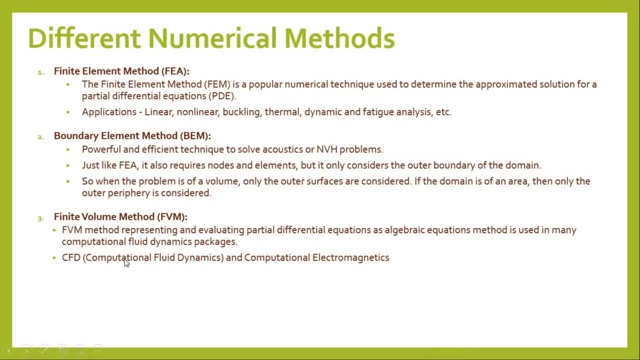 equations, as a algebraic equation method is used to many computational fluid dynamics packages. so basically it is used for a cfd or computational electromagnetics. the next: we use a finite difference method, like it uses the taylor series to convert the differential equations to an algebraic equations. this conversion process, higher order of terms, are neglected. 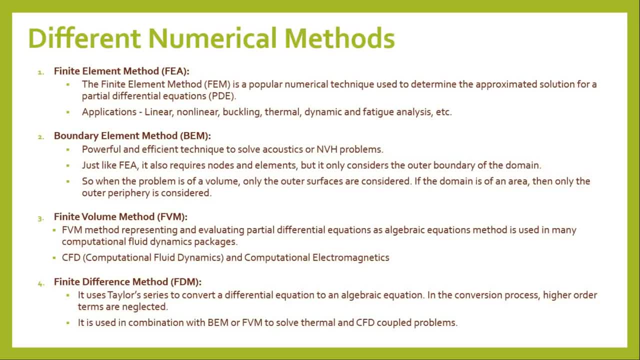 it is used in a combination with febm and feam to solve thermal and cmd couples. so all these 4 methods use the to solve the partial differential equations by using their different respective methods. ok, so most widely used, like fea, for cmd, like fem, these are the 2. 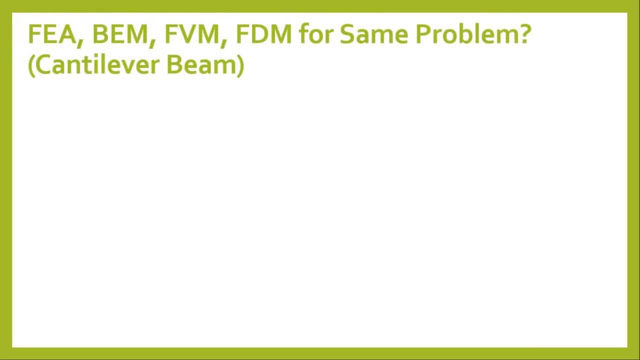 methods are most widely used to get the numerical problem solved. so now the next question will come like whether, al these four methods, is it possible to solve the same problem by using four meters? the answer is yes, but the difference in the accuracy. accuracy and programming is as 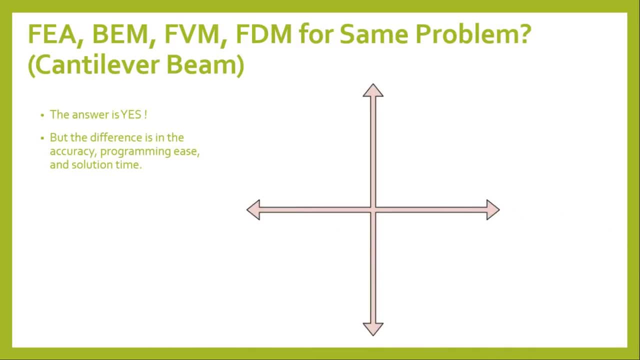 well as solution type of okay. so when we talk about FDM, it has the limitation with complex geometry, different material assemblies, different element combinations like 1d, 2d and 3d and the next when, when you talk about fe8, is quite useful. well, 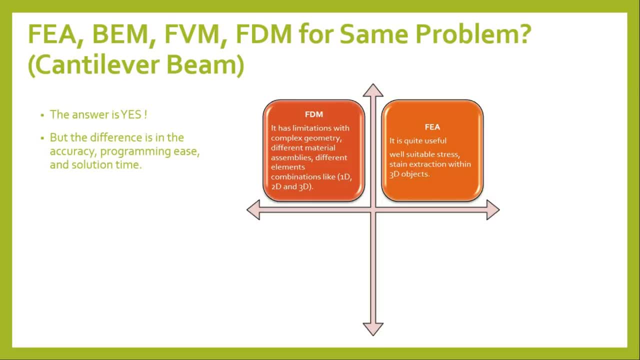 suitable stress extreme extraction within the 3d objects. the next method: like FEM, it has use of solving stress problem, but it is well suited for CFD problems. only convergences and equilibrium is quite natural in that case. and then the last year, FDM, or sorry, BEM, it will only consider the outer. 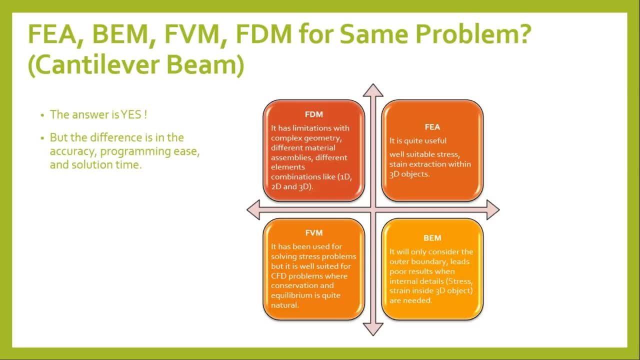 boundary and leads to the pure results when internal details, like stress strains inside the 3d objects are needed. so all this way, now the limitation. but you will definitely get the stresses or you can say the strain within the 3d object by using the FEM, which is most widely used. 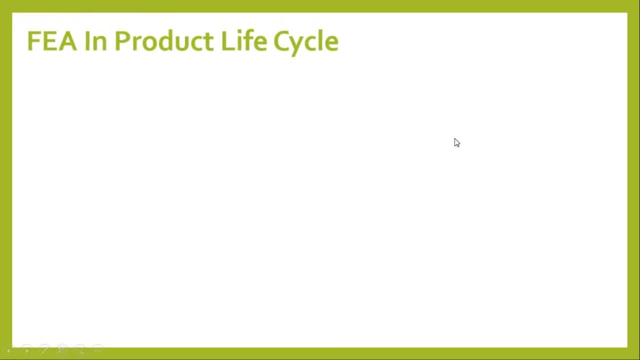 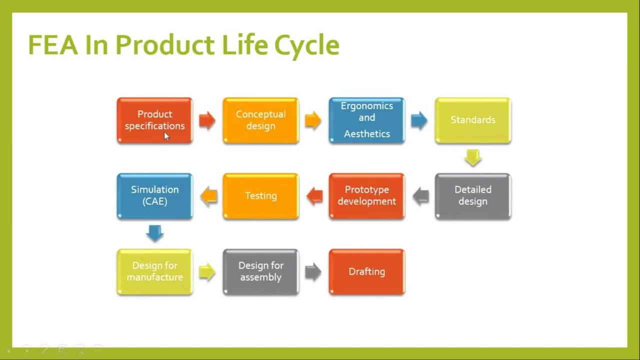 method. so now, when we talk about FEM, but where exactly this will lie FEM? so we'll discuss about FEM in a product lifecycle, okay, so here, basically, when we talk about product lifecycle, we first start with the product specifications, then your conceptual design will done. once the conceptual design will, then we will. 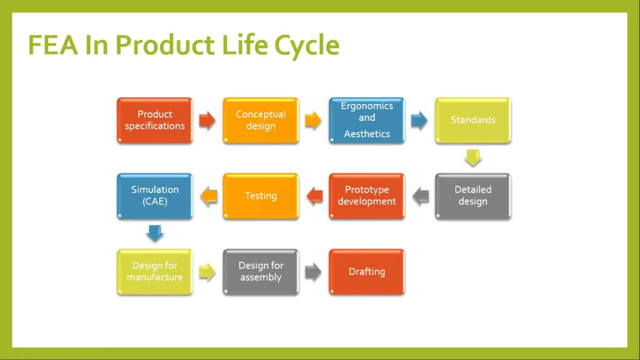 think about ergonomics as well as aesthetic look of that product, then we will do the standardization of standards, then we will go through the detail design. once our digital design is done, then we will further discuss about the prototype development as well as your testing for that respect to prototype. 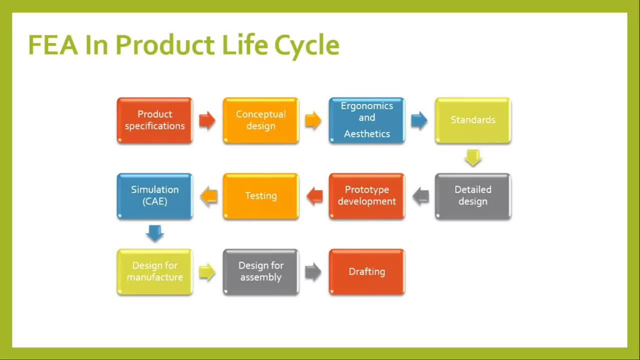 development. once the stating is done, then we will try to correlate that with in a similar, in a similar way. so simulations will come at this point of view. okay then, once simulation is, then, then we will go through the design for manufacturer, design for assembly, and then final step is drafting. so, as we saw, that simulation is will come after the. 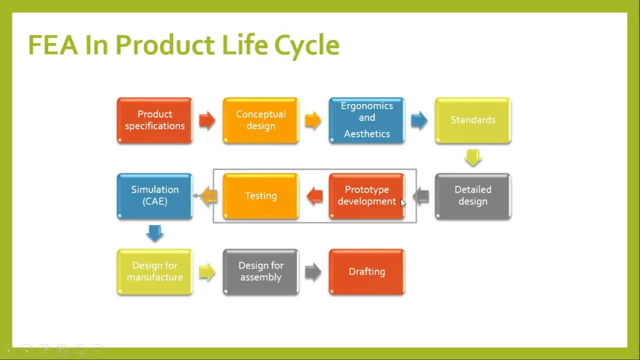 testing as well as prototype. but there are some of the cases or some of the industry which don't want to do the prototype and testing, so they just simply want to rely on a simulation. so they what they will do based on the detail, design, this directly go to the simulation phase and based on that, 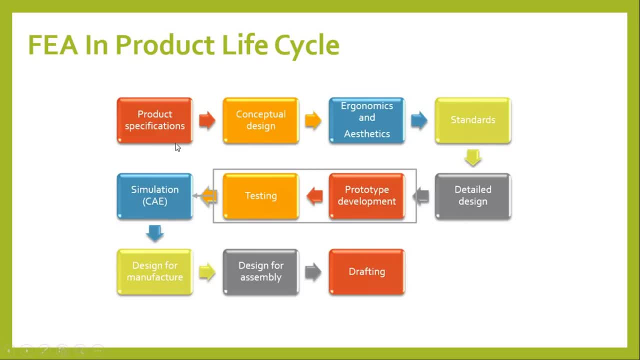 simulation or FEA, they validate their design and then they simply go to the design for manufacturer and design for our M3. take a example of pressure wishers like they: once they have design that pressure by using a standard- they don't want to do prototype- they directly go to the simulation phase and then once 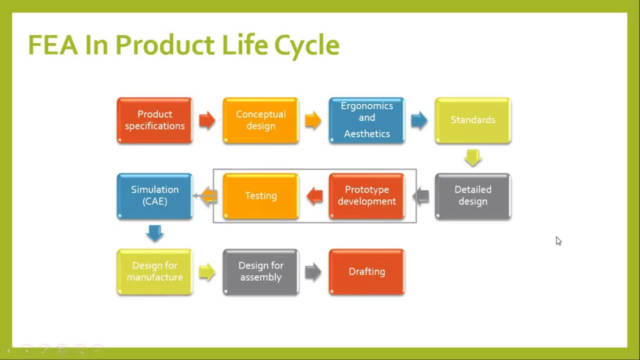 simulation is done, then they can go to the design for manufacturing and some. okay, so like that, you are a FA, I will come to the simulation phase and then, once simulation is done, then they can go to, or it is said, the mandatory in any product life cycle nowadays. now we know. 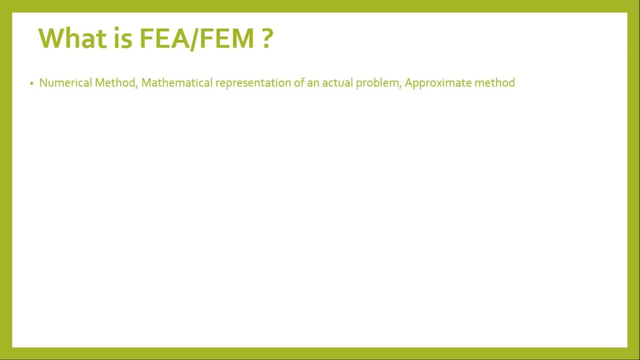 that if he is mandatory, but what exactly the FAA? so if he is nothing but your numerical method or mathematical representation of actual problem, or also, like it is approximate method, so we'll discuss that in more depth. like FEM, or you can say the F? E, when at 11 method reduces the degrees of freedom. 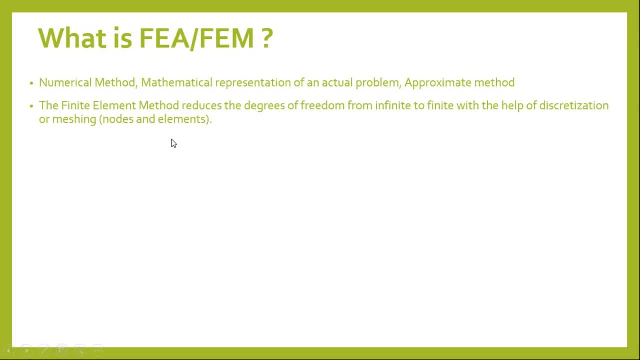 from infinite to finite with the help of discretization or a machine. so that is called nodes and elements. so basically, what it will do, it will reduces the degrees of freedom from finite to infinite. okay, so FEM, so what the F is, F is nothing but your finite. so reduces the degrees of freedom from finite to 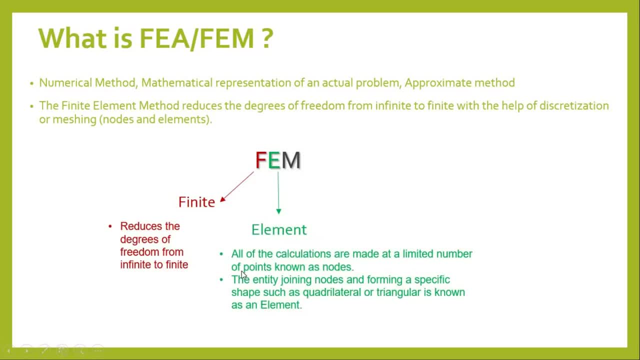 infinite element. he belongs to the element. so elements. all the calculations are made at a limited number of points, known as a number of points. so the number of points is the number of points that are known. the entity joining the nodes forming a specific shape, such as quadrilateral triangular, is known as a element. okay, and then the next term will. 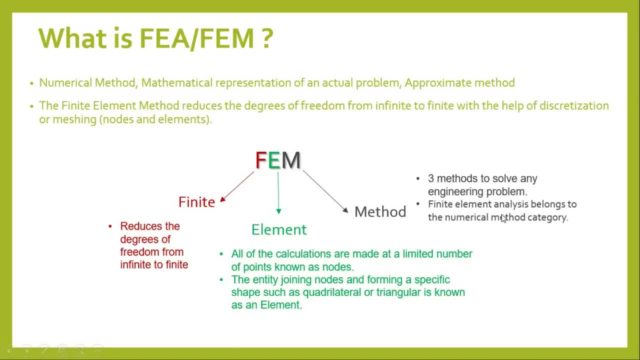 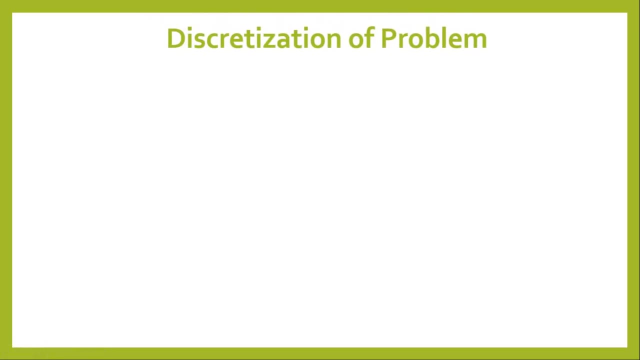 come your M. M is belongs to the method, so the three methods to solve any engineering problem, finite element analysis, belong to the numerical method category. so like that your FEM is, you can say the explained or illustrated. okay, then the next term, as we saw that a fee will down. but 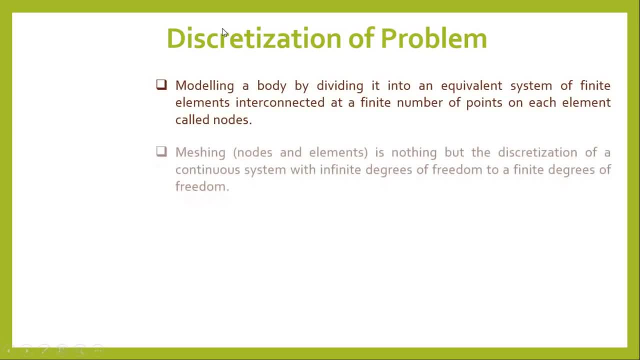 the discretization term is important. so what exactly this discretization? so modeling a body by dividing it into the equivalent system from finite elements interconnected at a finite number of points on each, elements called the nodes, meshing is nothing but the discretization of a continuous system. 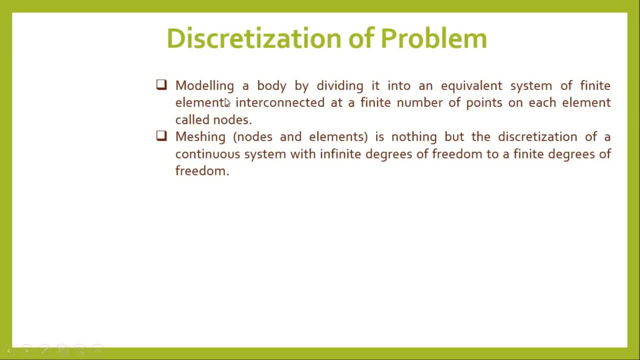 with infinite degrees of freedom to a finite degrees of freedom we will discuss. to one of the example like: consider the object. so, if you want to, this is what you are: rectangular, trapezoidal shape object and I want to split this object in a three different shape. you can see, this is one, this is another and this is third one. so all this. 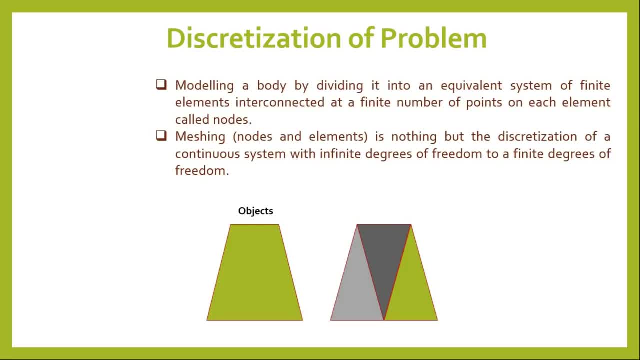 three from single object. we split it into the three object. that is called the discretization process and this three objects are nothing but your element. then from this elements, the outer boundaries, or you can say the outer portion, is nothing but your nodes. for this three elements you can call one, two, three, four, five nodes are: 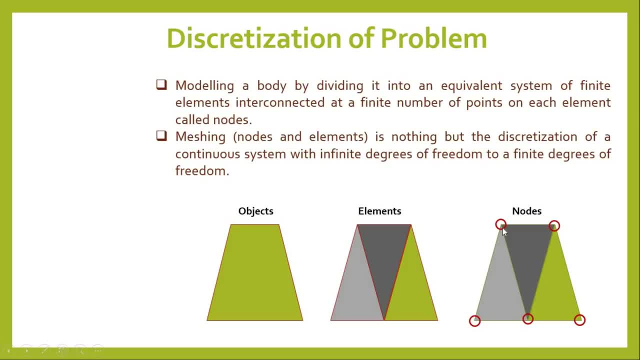 there. so basically, by forming this three element nodes you will get one elemental shape, so that is called element. okay, so like that, when we have any objects in the life cycle, when we discretize or when we split that object from infinite to finite, then that is the process is called as a discretization. so when we talk 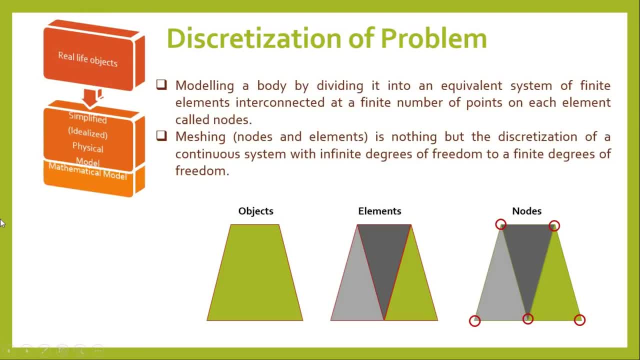 about real life objects, simplified or idyllic physical models, and when we convert that using the equilibrium mathematical model- consider any example of any blower or compressor which may have a real life or problem- then what we will do, we will discretize by using the creating a finite element model, by using doing a meshing for that. 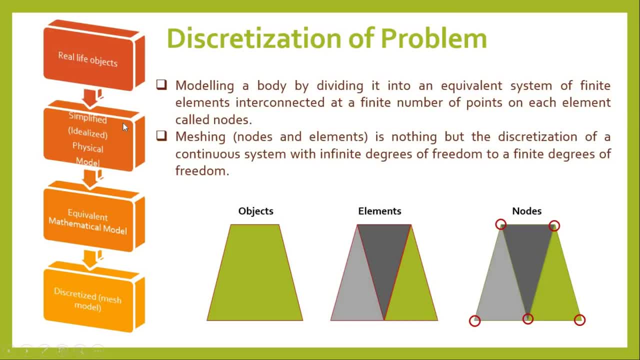 and then, once your meshing is done, we will move to the next part of the FEA. okay, so like that in any real life problem. you just need to simplify that idealized physical model by using equivalent mathematical model to get the mesh done. then the next term will come. 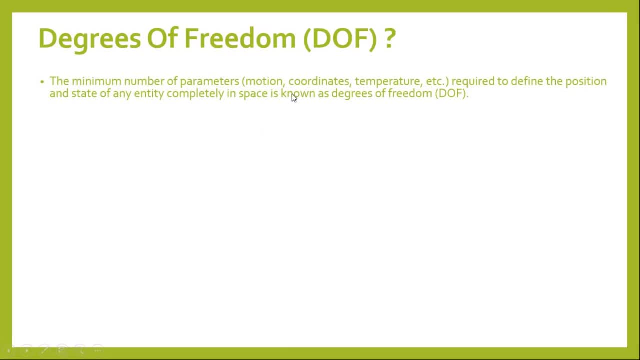 that is very important- degrees of freedom. so the minimum number of parameters, like motions, coordinates, temperature, required to define the position of any states, of any entity completely in a space is called as a degrees of freedom. when we talk about a single point right, consider a point a which. 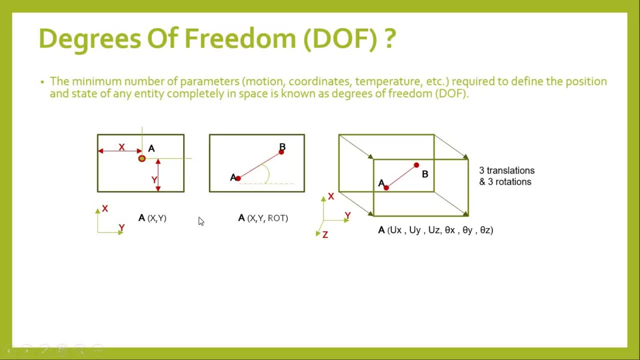 is defined by two parameters, like X and y. so this is the other thing, but you are two degrees of freedom for this define at this point, when we talk about the line, when the line will come, then there will be three parameter to define this line along. this for a point. 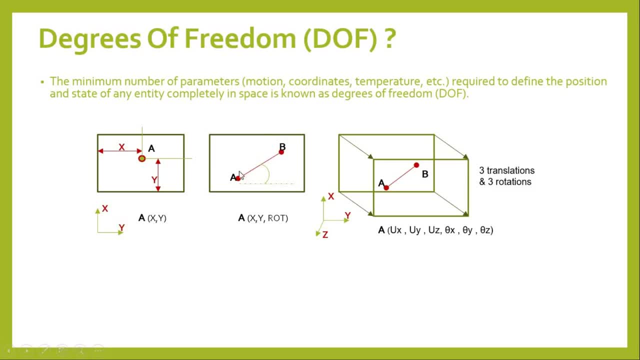 so X, y and rotation. suppose this line is like in a cubical kind of structure, so in that case we need at least three translation as well as three rotations to define this uh, a, b line. so that is like a, u, x, u, y, u, z. so displacement along x, y, g and rotation along x- y g, so like that six. 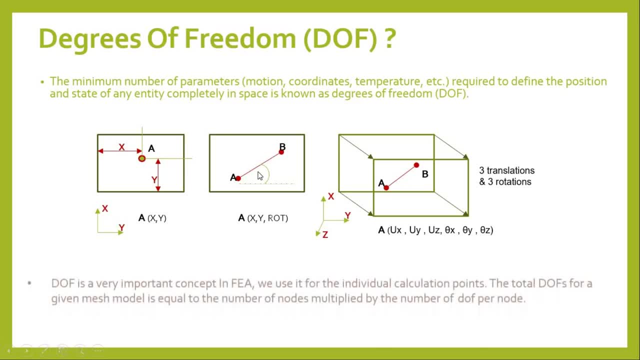 degrees of freedom will come into picture. okay, so the dof is very important concept. in fea we use it for the individual calculation points. the total degrees of freedom for a given mesh model is equal to the number of nodes multiplied by the number of degrees of freedom per row. 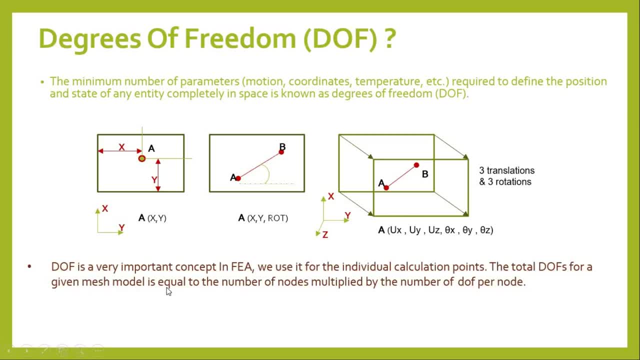 so basically we should know that the given mesh model is equal to the number of nodes multiplied by the number of degrees of freedom. okay, suppose there are like six degrees, uh, 100 nodes for this cube. so and having a six degrees of freedom for each node, so the basic equation for 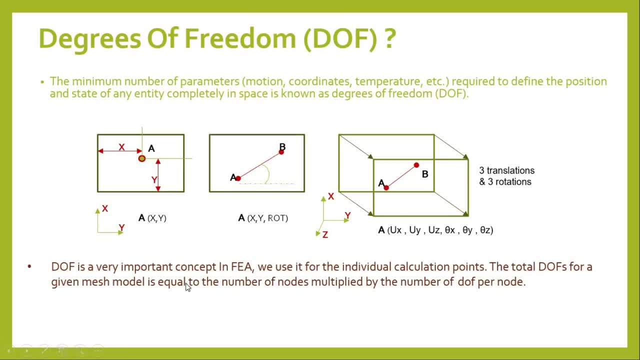 the number of nodes multiplied by the number of degrees of freedom will be 100. into this, six kind of thing. okay, so the number of degrees of freedom depends upon the type of filament, like 1d, 2d or 3d, and the family of the element, whether these are like thin shell, plain shell, stress membrane. 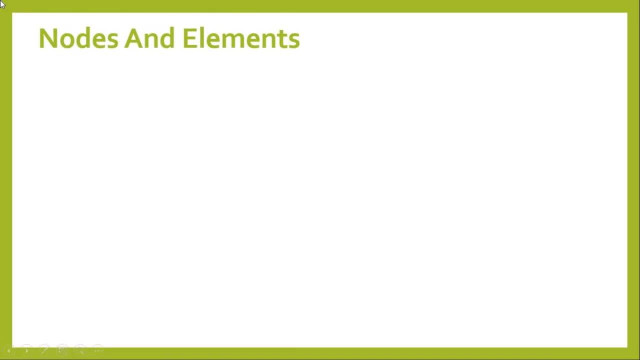 elements and as well as the types of analysis. okay, we'll discuss this in later slide. so, the nodes and elements, and we already saw, uh, nodes and elements. the total degrees of freedom for a given mesh model is equal to the number of nodes multiplied by the number of degrees of freedom. 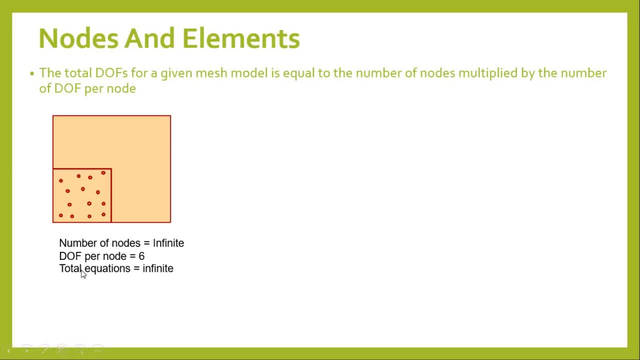 consider this rectangular object in this rectangular patch. so here, like, number of nodes are infinite, total degrees of freedom are six degrees of freedom. so the total equations are like infinite into six. so number of nodes into degrees of freedom per nodes. so here it is infinite, right when we make it from infinite to finite. 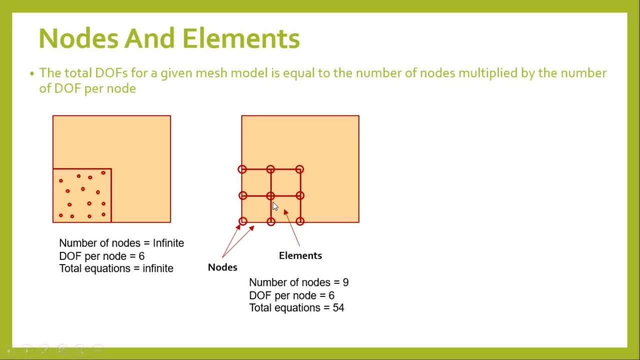 using the one, two, three, four, mode, uh, four elements, which is having the number of nodes nine and six degrees of freedom per node. so the total equation will be: nine into six is equal to 54. okay, so what we did, from infinite to finite, we made. so we got some equations. so they are like: 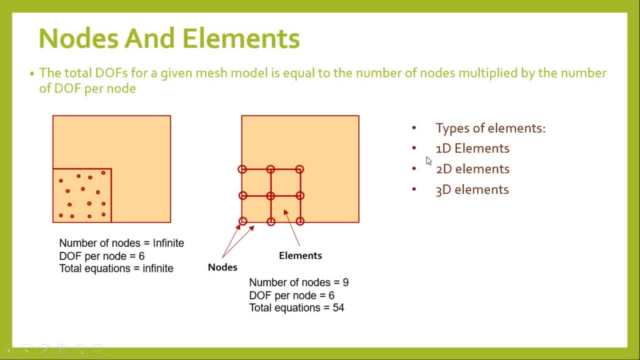 three types of elements: 1d elements, 2d elements and 3d elements. okay, so the finite element method is basically based on three component per unit, 12 and 6 limit\. now, first one, to go into understand the final use case that we used for maf違う. 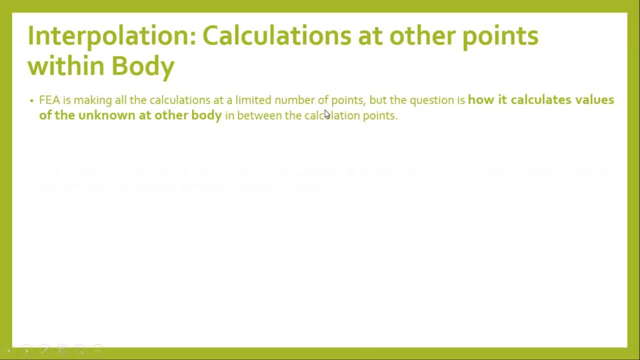 so here was our mathematical form. you had the values of, you can at limited number of points. but the question is how it calculates the value of unknown at the other body in between the calculation point. so this is done simply by using the interpolation. consider the four quadrilateral element. 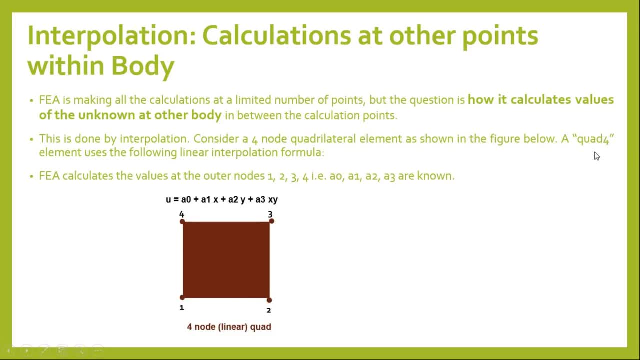 I shown in figure, so you can consider this. a quad four elements uses the following interpolation equation: so you can see this. this is nothing but your interpolation equation. suppose you want some of the displacement at point. this is so you can use this equation: a 0 plus a 1 X plus a 2 y plus a 3 x y. so if he 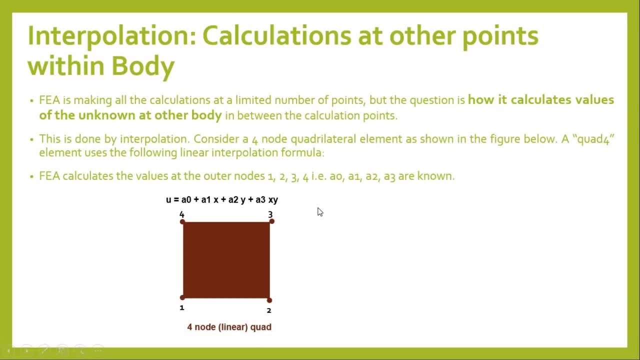 calculates the value at the outer nodes one, two, three, four, zero, right so from this node. so if you use this equation, you will get the displacement or your results at other than this calculate nodes. now, this is what the eighth node parameter got, so for that you can have a equation like this: a, 0 plus a, 1, X plus a. 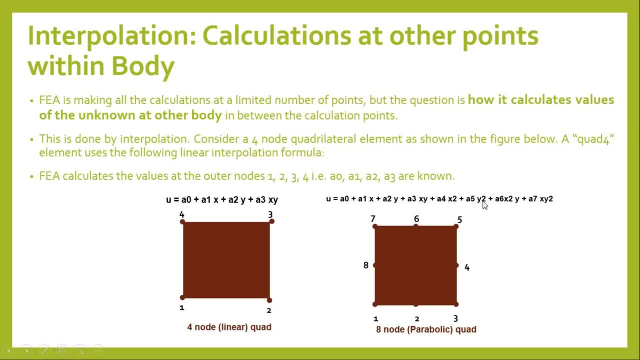 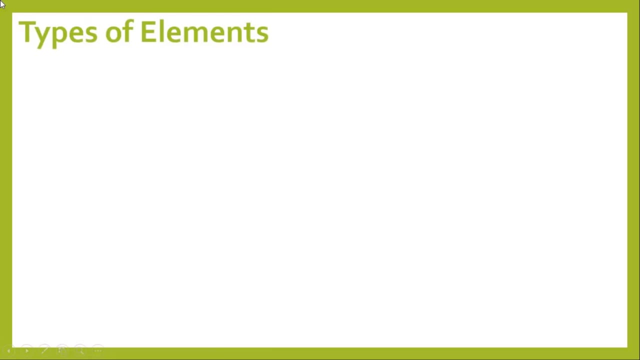 2 y plus a, 3 x, Y plus a4x2 plus a5y2 plus a6x2y plus a7xy2. so like that your parabolic node chord interpolation equation is used now once your interpolation is done, then, as we saw that there are element, 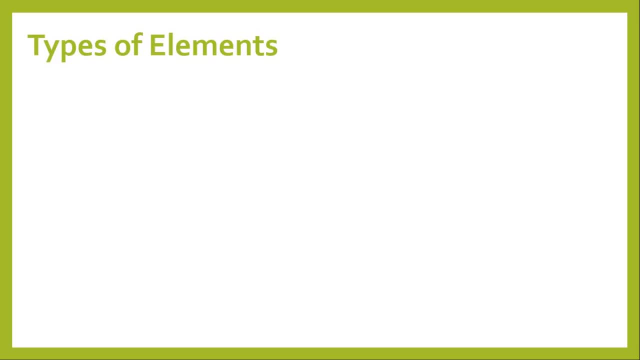 terms. so what are the different elements are available in the commercial software, so we will discuss that in the slide. so like there are three major element types like 1d, 2d, 3d and other, so 1d are like one of the dimension is very large in comparison to the other two. 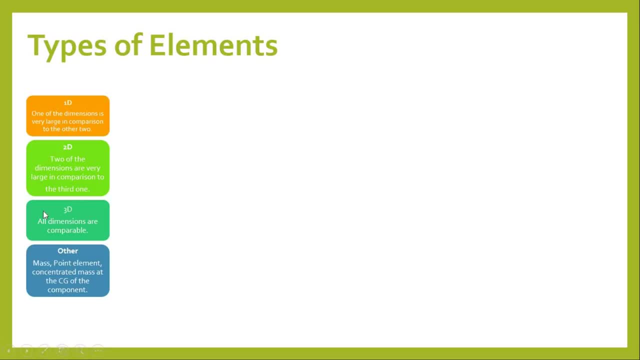 2d, like two of the dimensions are very large in comparison to the third one, and in 3d, like, all dimensions are comparable. so other than this, there are also that few elements, like mass point elements, concentrated masses of the cg, so this element suppose. consider the: 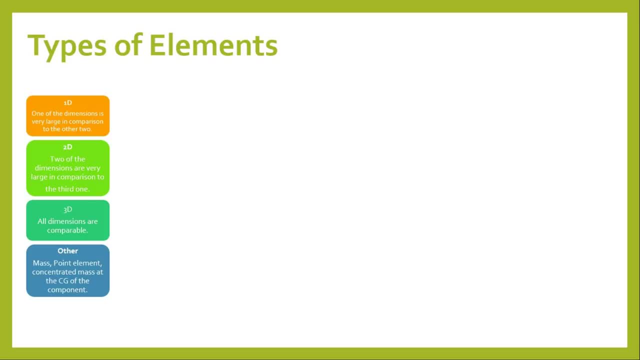 example of a compressor base frame, right? in that case, if you want to simulate the base frame, then you don't want to consider the complete geometry, like compressor, motor, air, and so what you will do? you will simply idealize that components by using a mass element and that simply connect. 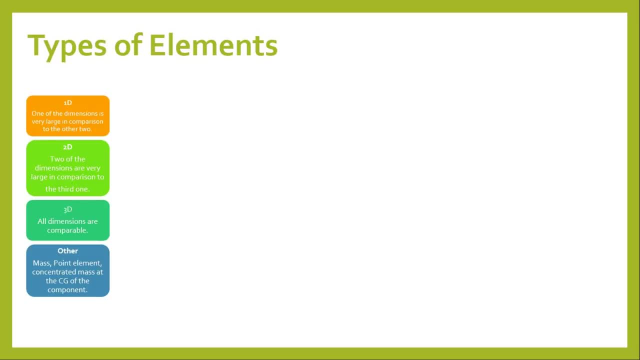 that mass element to the mounting location. so these are come under this category. so the 1d element, like shapes, are line elements. so the types like rod, bar beam, and the examples are like long sharp beam, pipe pin joints when we talk about 2d. so shape will be your quad tria, r, tria and the elemental 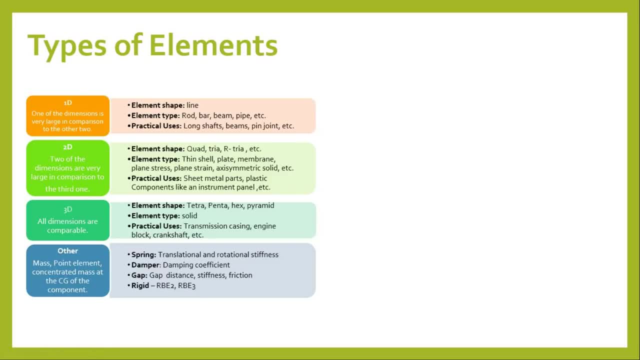 type like thin shell plate membrane plate stress, plane strain and axisymmetric models, so like that your all 2d elements will lie under this. so the examples or you can see the application, like thin shell plate, membrane stress, these are the element type, but the practical uses are. 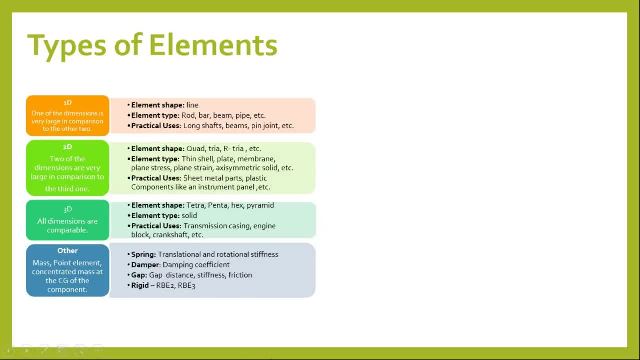 like sheet metal parts, plastic components and instrumental panels. so the basically the sheet metal parts. you can take the example of bumper of your car, so that will come under this 2d category. when we talk about 3d elemental shape, so that will be like tetra, penta, hex. 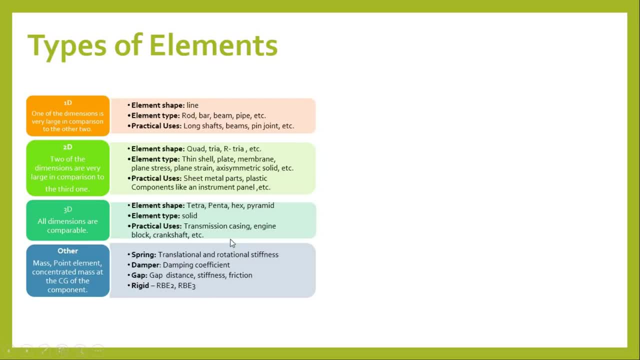 pyramids. so element type will be like a solid. so the transmission casing, any engine block or any complex geometry like kankshaft, so that will lie under this 3d category. okay, then next time we will come like as we said earlier, we will come to the 3d category. so 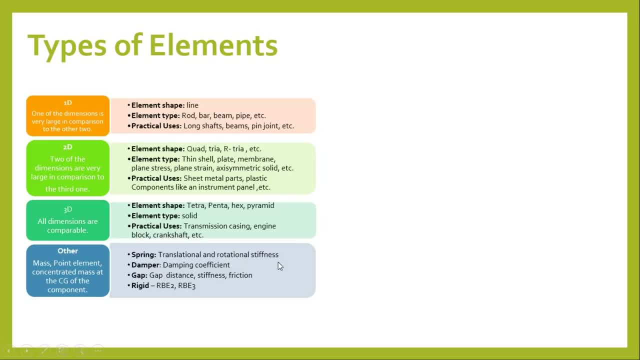 as we saw about other categories. so that is nothing but your translation. and rotational stiffness dampers, like damping coefficient. you can define gap distance stiffness, friction, and rigid like rb2, rb3, so this will come under this category. so they are like. two major softwares are available in the market which are widely used, like abacus and ansys. so in abacus you 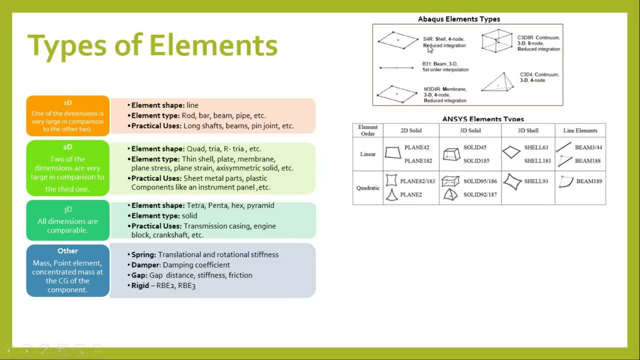 can have an element type designation like s4r, shell. 4 nodes reduce integration, d4 nodes b3, 1 like 1d element, so b beam, 3d first order intel pollution, so m3d are membrane, 3d, 4 node three, centrifugation. when eight node it reduces integration, so it is defined by c3dr when 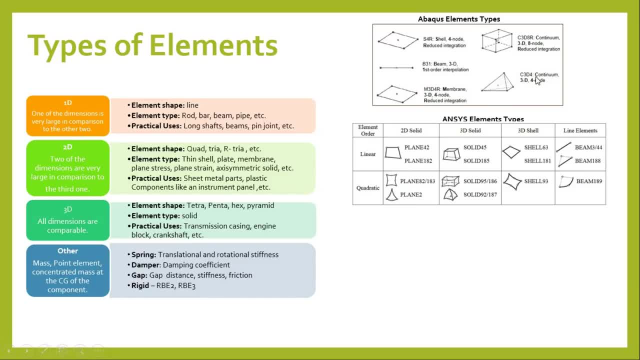 it is like your tetra, so it is like c3d4, so like these are the major element types used by abacus elemental library and when we talk about ansys, epidion, so there it is like for linear 2d, plan 42, plan 182.. so this is the 3d type. so this is the 3d type. so these are the major element types used by abacus elemental library and when we talk about ansys, epidion. so there it is like for linear 2d. you can have element type designation like s4r, shell 4, node, reduce integration d4. 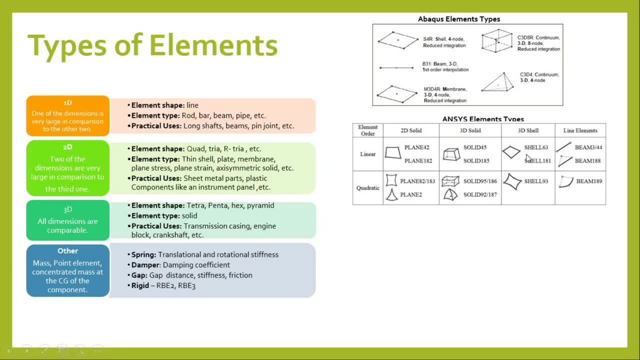 or sph3 node, reduce integration in b1 and b2. well, in the atta you also can have element type designation like of 3d solid 45, solid 185. similarly, shell 16, shell 63, 181, beam 344, 188, so, and then when we talk about quadratic, so there you will find like a second order. 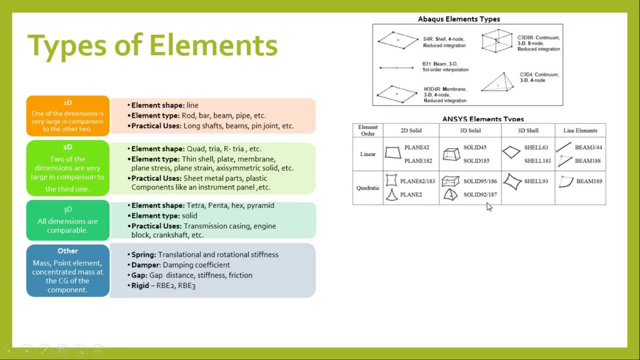 plane to plan 82 for 2d solid, 3d solid line 95, 186, 92, 187 and 3d shell like a shell 93 beam 189. so like that elements are used and there are a lot of parameter which are used. 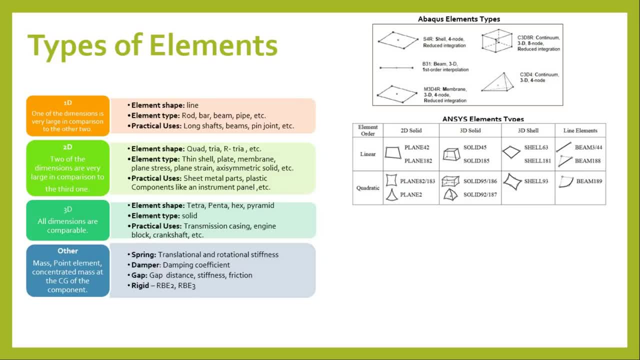 in that selection- and that is actually what we are going to talk about in the next lecture- are available in abacus as well as ansys elemental library. we need to go through this, so this is one of the example of types of elements you can consider. this is nothing but your solid block. 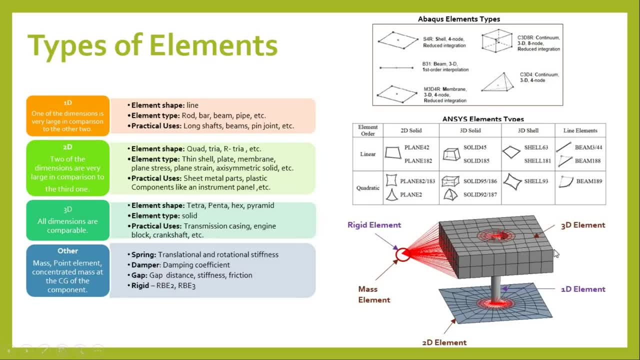 which is connected with this plate. so this solid block is meshed using solid elements. that is called 3d elements and this is shell is meshed by using 2d elements. you can see between this. these are: both are connected by using beam element, so that will come under the 1d element, right and these: 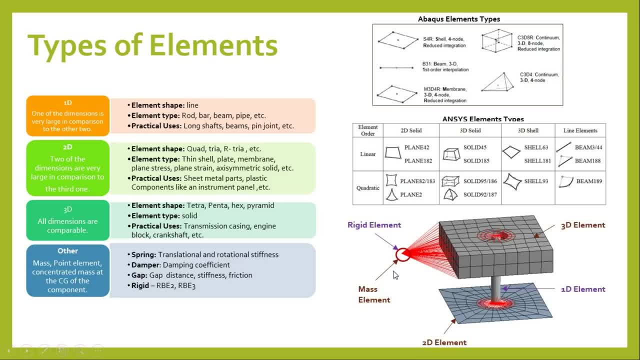 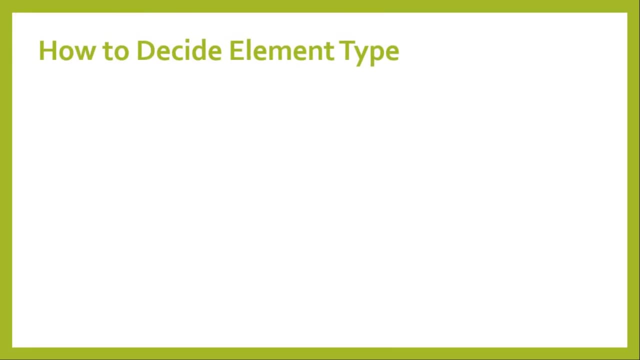 are like, as we saw about discuss mass idealization. so you here you can put a mass element and these are that rigid elements which are connecting to this 3d. okay, so the types of elements are very important when we talk about fea now, once your element type is selected. but there one thing will: 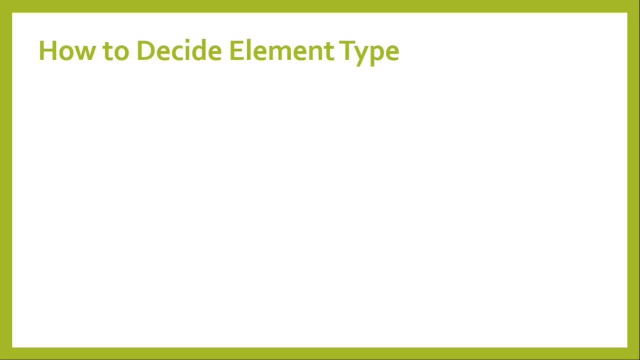 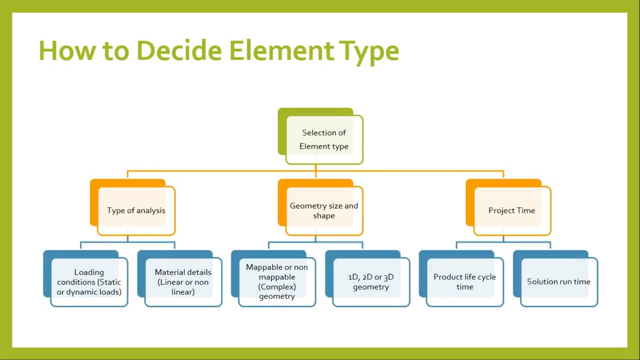 come into mind how to decide the element type. so in that case, there are few things which will come into mind. based on that, you can define element type. so like three major things: types of analysis, your geometry, size and shape, as well as your project time. so when we talk about types of analysis, so there are like loading condition. 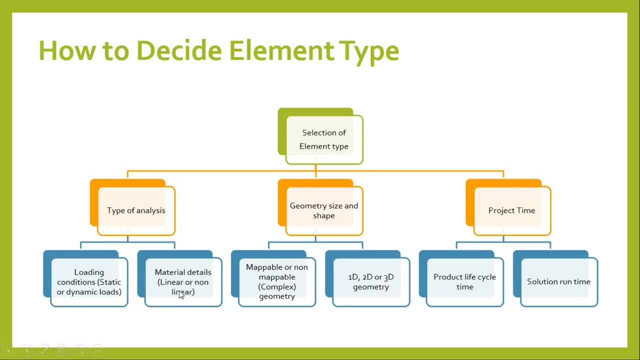 whether it is static or dynamic load and the material it is, whether it is linear material or nonlinear material. so basically, linear, you like your steel or any other nonlinear material will be like your plastic. non metals are there and geometry, size, shape, like a mappable, whether it is mappable or non-mappable, and you are like whether it is 1d. 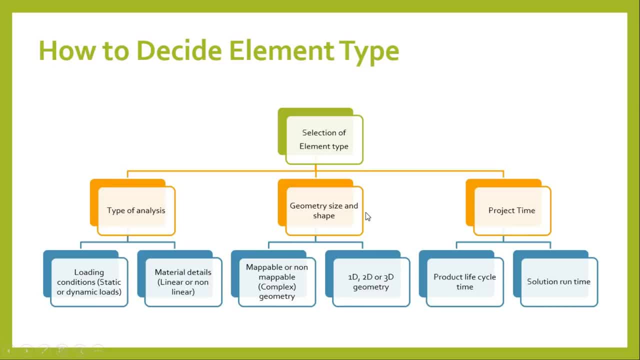 2d or 3d geometry, so like that the second term will come: geometry, shape and size. the another term is like project time, so the products, life cycle time and solution runtime, basically when you are suppose your product is belongs to the automobile category, so in that case we always 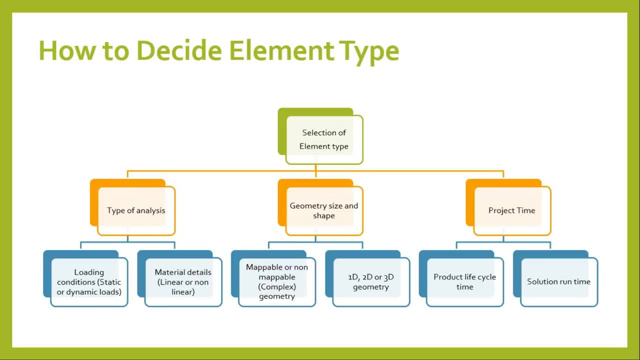 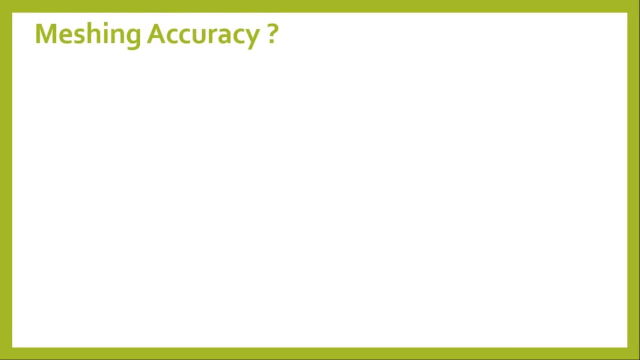 need to think about the life cycle time, right? so based on that also, you need to think about the element type. okay, so these are the three major things. if you know these things, then you can definitely decide the element type. then, once your element type is defined, then you need to think about the accuracy. so the we will. 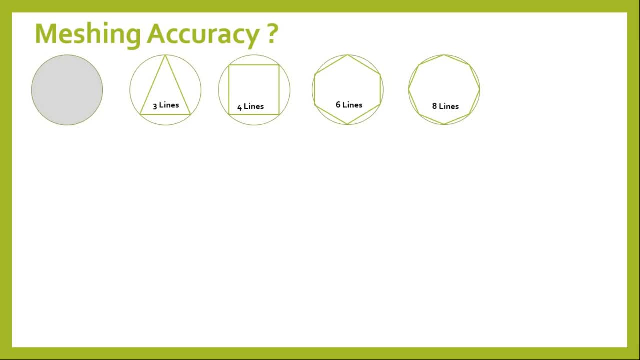 discuss that how to decide the machine accuracy. consider: this is the sphere, your complete sphere, right? so if you split this sphere by using three lines, four lines and six lines and eight lines, so the eight lines will represent the more accurate shape of this sphere. so, similarly, if you put 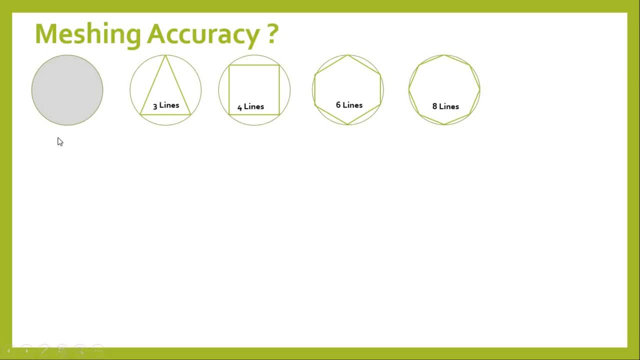 few more lines you will represent, the more- uh- your accurate shape of this. so definitely, if you increase the number of lines, you will get the more accurate shape of this. so, similarly, in case of meshing also, it will be like this, only we will discuss that through this t-pipe example. 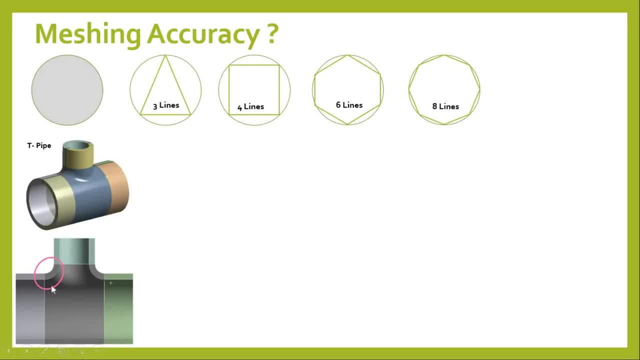 so this is what, uh, ourτ-pipe will consider. this is nothing but your bend radius. so we will consider this much portion and we will try to match this point, uh, this curvature, or fill it. first we will try to put two elements. then, if you see, here it is not more accurate or not capturing proper profile when we put. 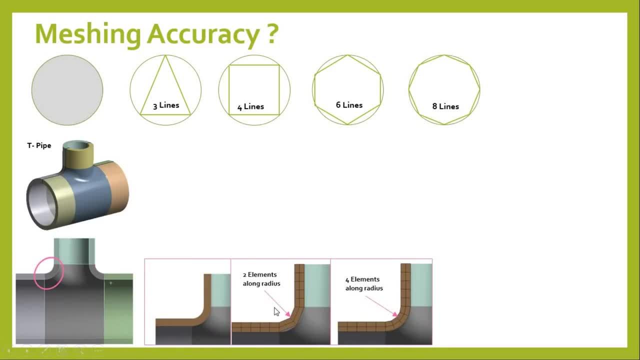 few more elements, it is having a better compared to the two limits. when we put few more elements, more elements like six, eight elements, then it is like capturing the curvature properly, right, and here, if you put more finer than that, so it will be more accurate compared to the eight elements, right. so it is similar when we put the 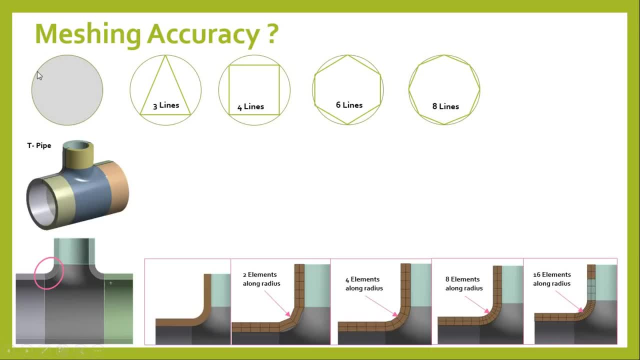 increase the number of lines, you will get the more accurate sphere. if you increase the more number of elements, you will get able to capture the mesh lines, curvature. but here one question will come into our mind, like how many elements then we need to put so there also your engineering judgment will come. 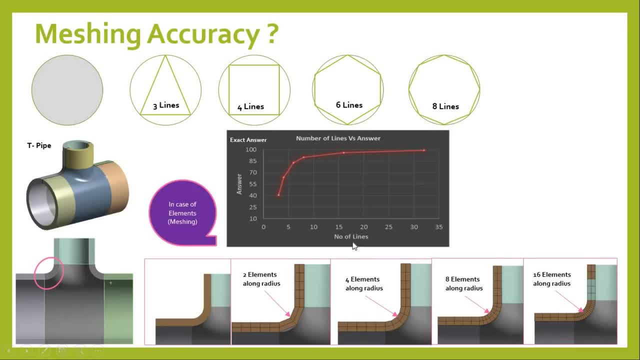 we will discuss this through this graph. horizontal line with shows the number of lines or elements and how. vertical line shows the answer. when we increase the number of lines, it will give the more accurate results, like 100, suppose. if you put like 32 or 30 more than 30, it will give 100 percent accurate result. 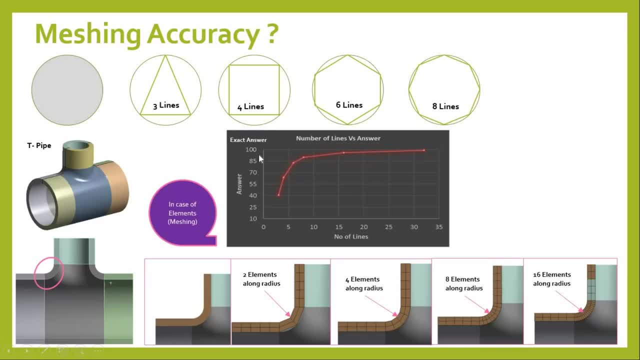 but if you put like 20 to 25, it will also give the 95% of accurate results. at the same time, it will reduce the times to get the mesh done. okay, so we need to think about these things like more number of lines or more elements, more. 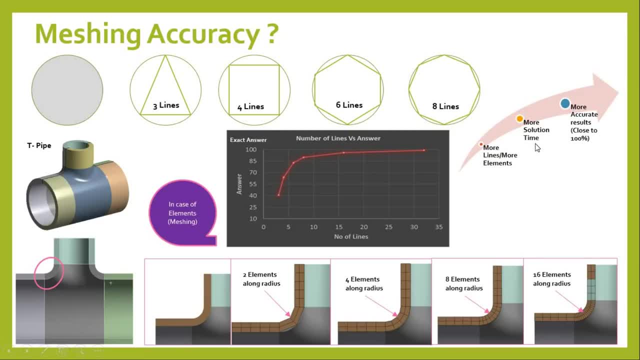 solution time, 100% accurate results. but nowadays we don't want 100% accurate result because most of the things are time dependent. so in that case we need to do the moderate mesh, we need to do the less solution time and then we at least we need to get the results by 92- 100% accurate. so this is the most 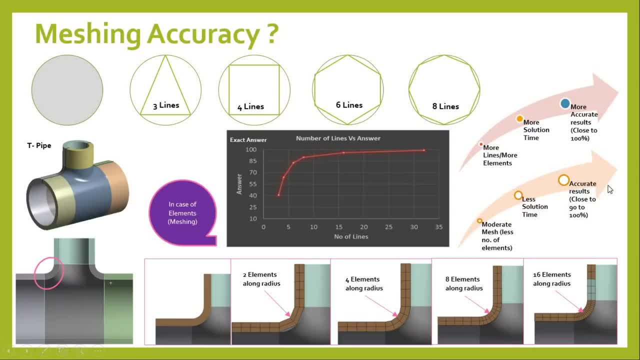 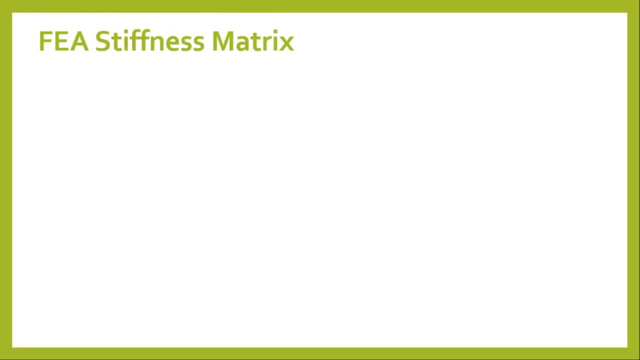 widely used methodology nowadays with the industries, because if you put more number of elements, ultimately it will increase your efforts and time, okay, and also the solution time to get those equations. all will increase. now we will talk about the Fe's stiffness matrix. so like we saw the different element types. 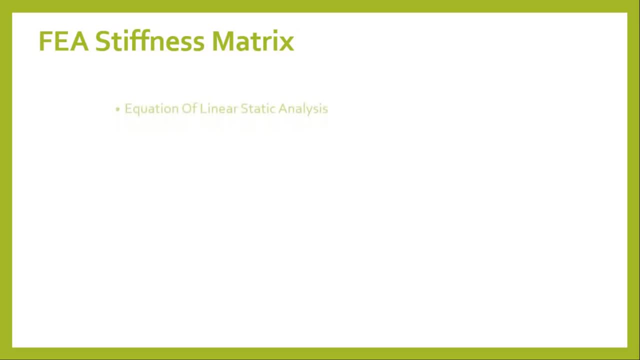 and this, then the linear equation, or you can say the equation of linear static analysis, is defined by this basic equation, as all of us know that F is equal to K into D. so here, F is nothing but your forces, is really unknown, and K is nothing but your steepness, this characteristic property of the element. 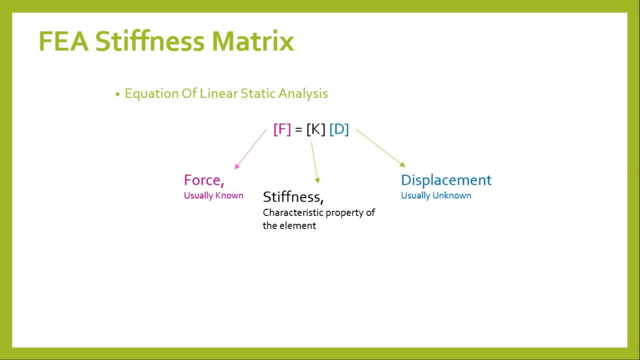 and these you are nothing but your displacement, so easily unknown. if you know any two properties, like: if you know the force, you can definitely calculate the displacement. if you know the displacement, you can definitely calculate the force. okay, so this is the linear starting equation which we calculate: the F, a stiffness matrix. first, we can formulate the stiffness matrix. 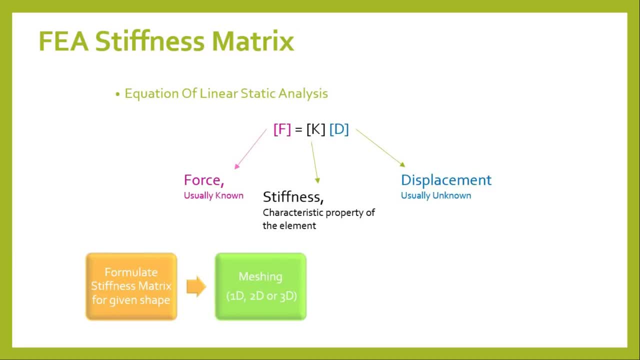 for a given shape. then once it is done, then we will do the meshing 1d, 2d, 3d. then we will get the solution done, or solution equations. then, after solving that equation, we will try to get this unknown. okay, so like that, the process flow is there. first you need to formulate. 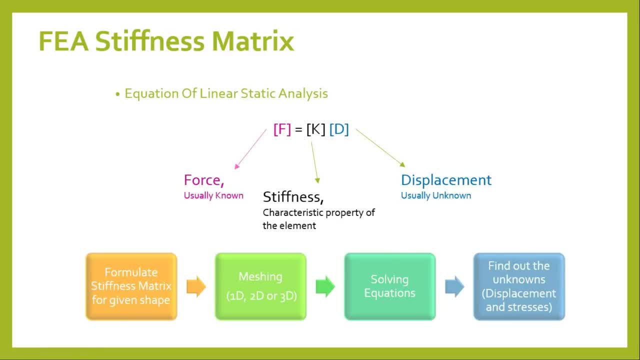 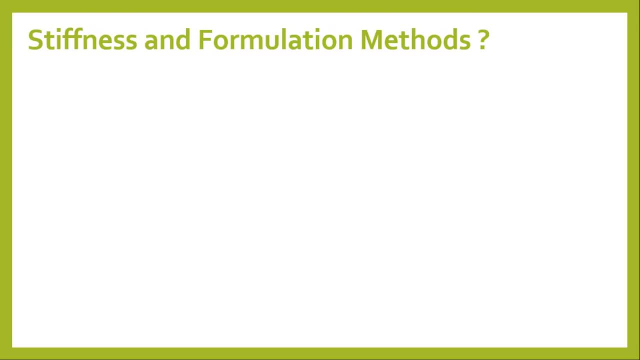 stiffness matrix, then meshing, then solving equation and then find out the unknown. so when we talk about stiffness matrix, so the stiffness and formulation methods are coming to mind. so we'll discuss that. steepness K is defined by force per unit length. so steepness is equal to the force required to produce. 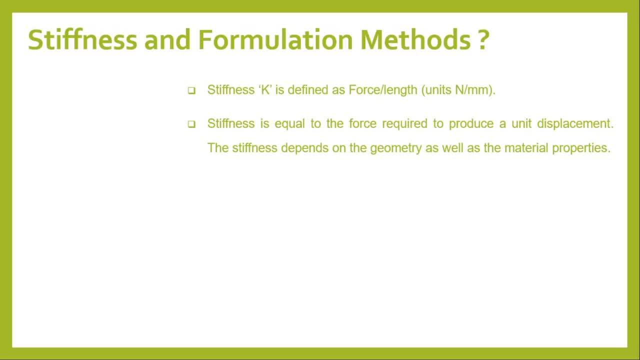 the unit displacement. the steepness depends on the geometry as well as the material properties. okay, so consider the three rods having a three different materials. we had applied of same pool force for a three different metal. first is cast iron, second is mild steel and then aluminum. so all these three we are. 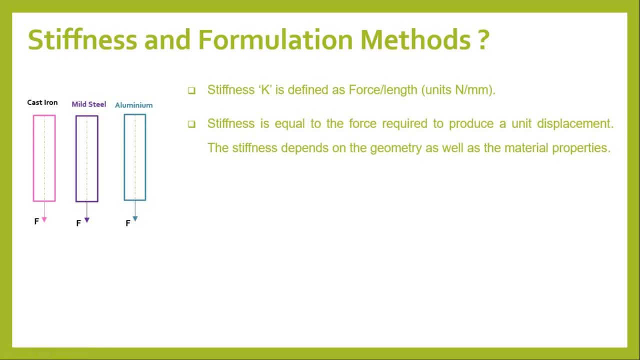 applying the same force. but here question will come into mind, like which of these three rods having a higher steepness? so here, as we saw that steepness is very high. so we are applying a higher steepness. so here, as we saw, that steepness is very high. so here, as we saw that steepness is very. 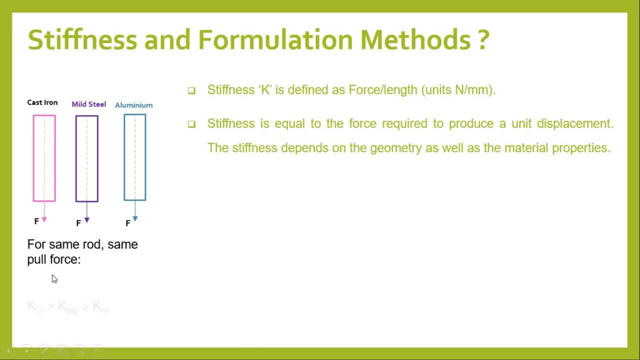 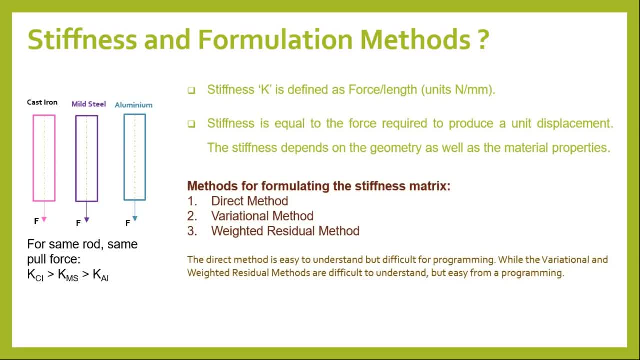 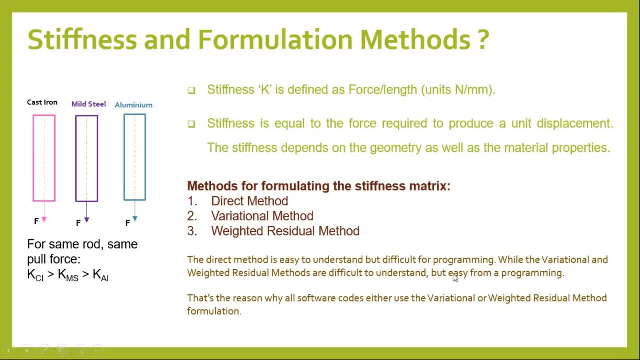 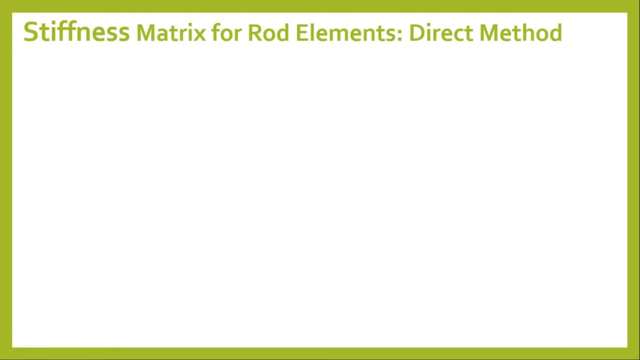 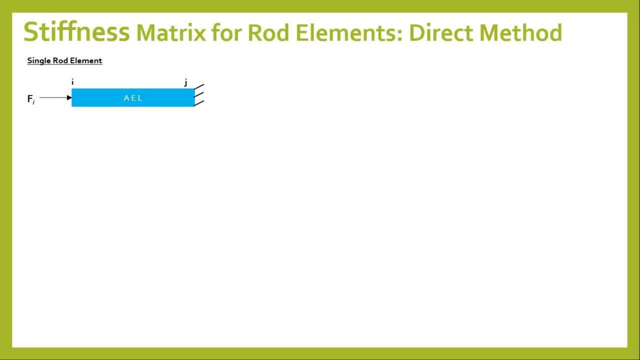 elements which may consist of two nodes, that is, I and J, which is fixed at one end and other end, at I node, the force is applied. so A is nothing but your area, E is Young's modulus and L is your length. so all of us know that there are like: 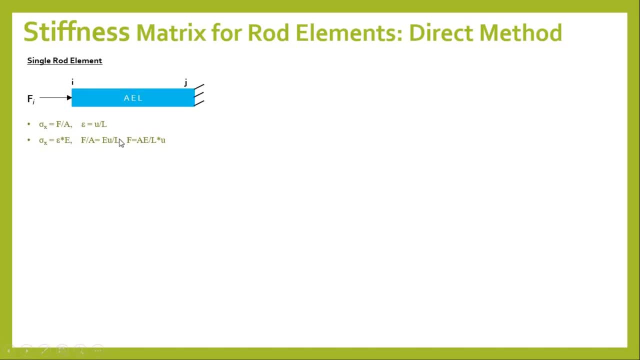 some relation between stress strain. so based on that we will try to get this force value. stress is equal to force per unit area and strain is equal to change in length per unit original length. so from that we will get one equation that is like: F is equal to AE by L into U, right. so now we will try to use some. 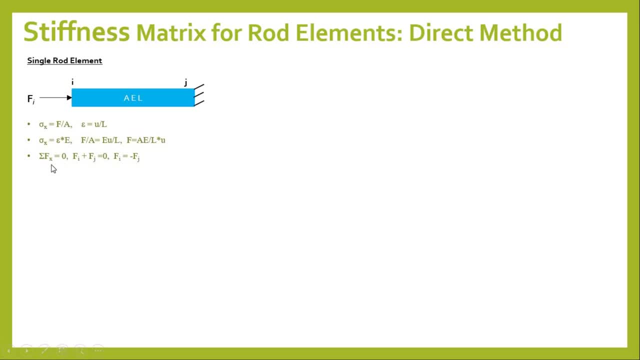 equation, algebra equation- like summation of forces, is equal to 0. so if summation of Force is equal to 0, then we will try to find out. F I is equal, sorry, F I plus FJ is cut equal to 0, so from that fi is equal to minus fj. now consider a case one where ui is equal. 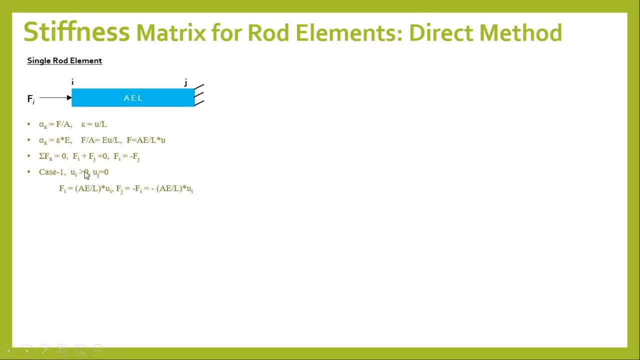 to 0 and uj is ui is equal to greater than 0. this point is greater than 0 and this is your fix one, so 0. so fi is equal to ae by l into ui. as we know that fi is equal to this one minus fj, so we will put a minus fj value over here, so that from we will get minus fj. 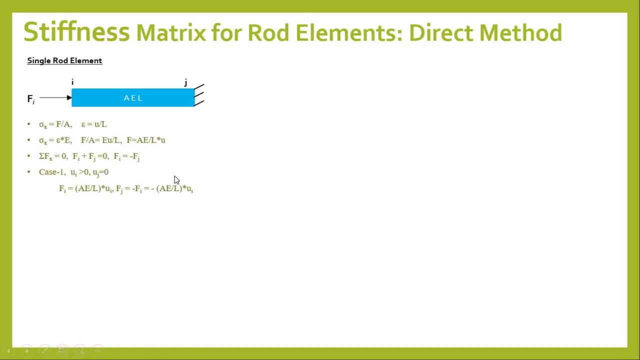 is equal to minus fi is equal to minus ae by l into ui. so like that, when we consider another case right, when we will consider this end is greater than 0, on this end fix, we will get the other alternative equations for fjs. so these are the two cases from these two. 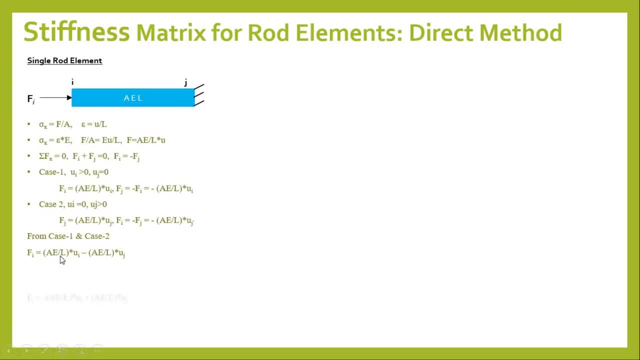 cases we will get the two equations: like fi is equal to ae by l into ui, minus ae by l into uj. so you are like ae by l is constant. so based on that we will try to form ae by l, this stiffness matrix. so if these are like force matrix- fi, fj having 2 by 1, and we will 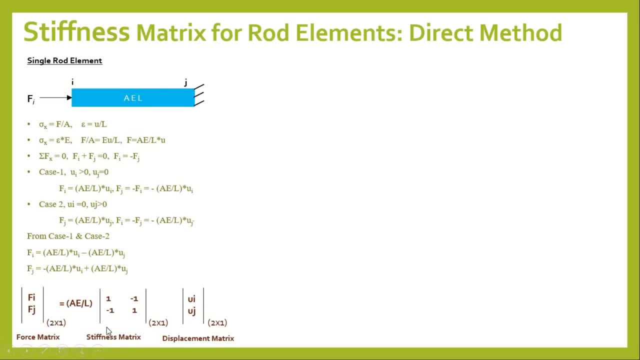 keep this common ae by l, and from that we will try to write stiffness matrix 1 into minus 1. minus 1, 1. this is also 2s to 1 and here your displacement last term, that is uj ui. so like that we need to form a stiffness matrix like: first is your force matrix another. 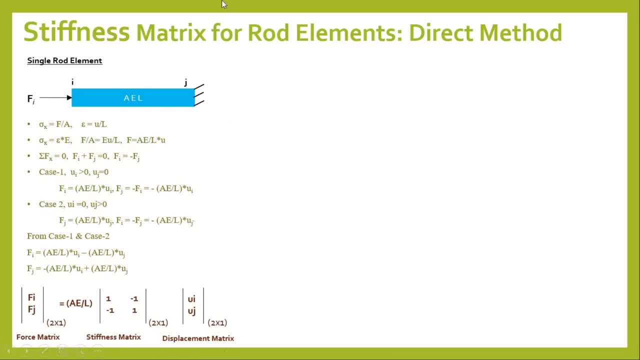 stiffness and then displacement, f is equal to k into d. okay, similarly, when we consider it to consider a case of two rod elements, like there are two rod elements having a different, different characteristics, defined by one and two, we, if you apply, pull force over here. first step, we will try to get us free body diagram right. 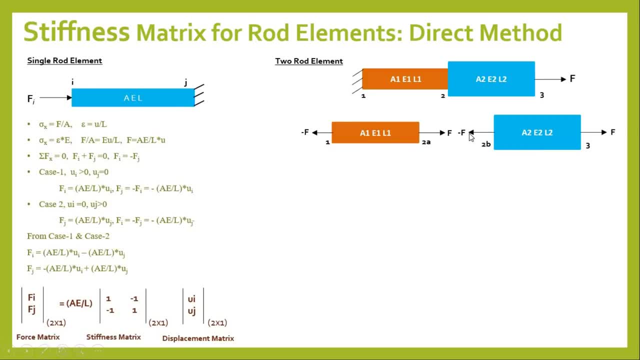 so we will try to get free body diagram for this f minus fmi, and here like f because it is fixed. so we will get some reaction over here. based on that, we will calculate these forces right now. similarly, we will try to find out these terms from this: rest and equation: what? 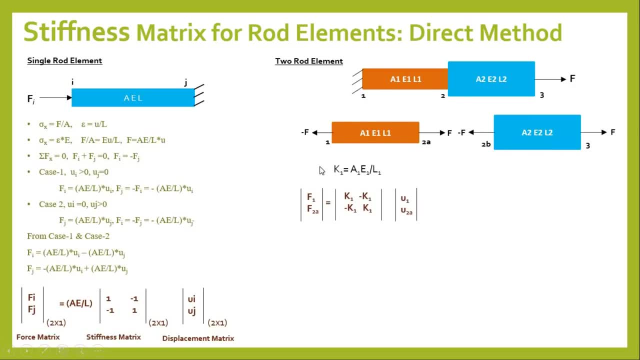 we saw in two rod element. so we will get the stiffness matrix- or you can say the force is equal to stiffness- into displacement like this: here: k1 is equal to a1, e1 by l1, so this term, what we discuss earlier, similarly for for this rod also we will get similar kind. 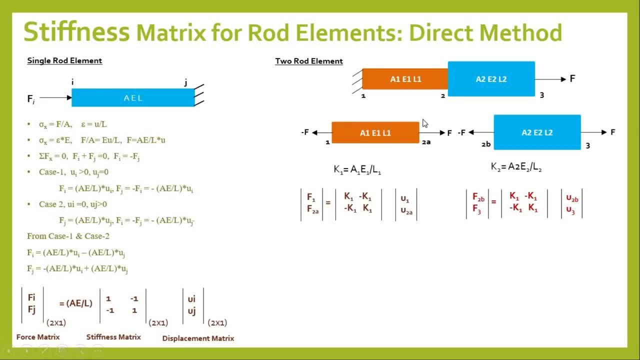 of matrix. so We will try to match these two matrix, try to sum from these two. some matters will get a. one matter is like if you add f1, f2a plus f2b and last one is f3, so from that we will get this matrix and similarly here. first displacement u 2a plus u2b is equal to u3, right? so when 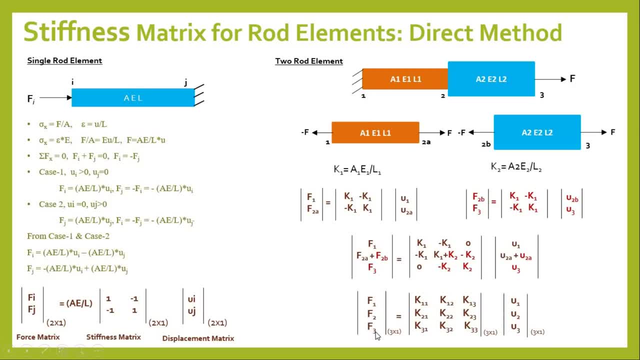 we add, we will get some another matrix like f1, f2, f3. these are the forces value and these are the stiffness value, and this is what you are discussing. yeah, right, and then here we displacement. So likewise, we need to formulate the matrix X. First, we need to formulate: 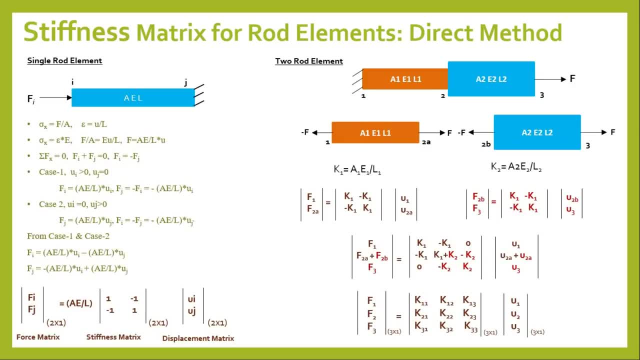 the equation and then from that equation we need to form the matrix X. So then this FEA will going to calculate based on this matrix X. So if there are 3 elements, similarly we need to do 3,, 4,, 5, whatever the raw elements are there. Likewise we need to form this: 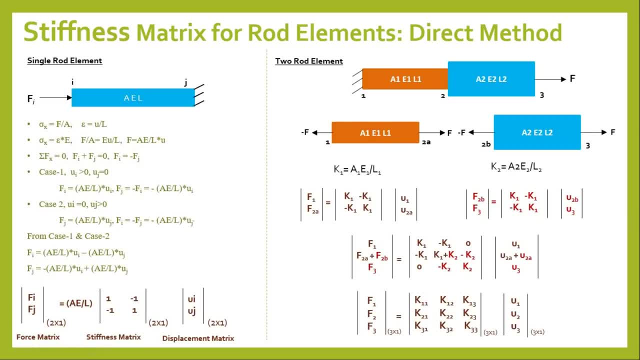 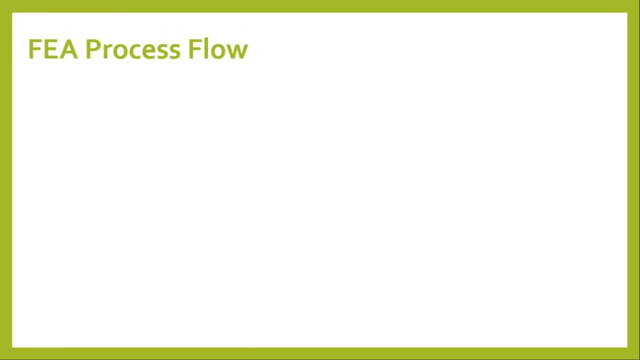 matrix X. Now we will discuss about the FEA process flow, as all of us know that FEA is one of the method to solve the engineering problem. but what are the processes involves in this? So first process is nothing but your pre-processing where, like geometry, clean. 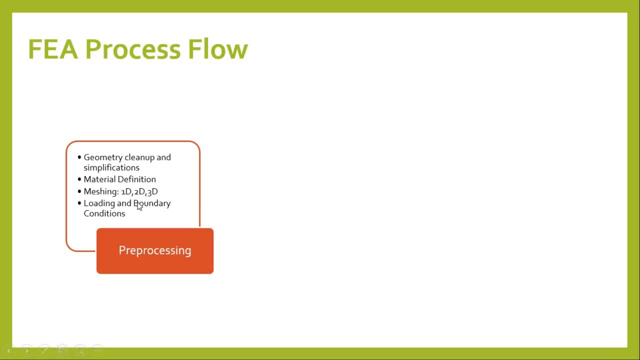 up and simplifications: material definitions, meshings 1, 2, 2D, 3D, loading and boundary conditions. So like first phase will be, for you need to create your FEA model for the solutions. So that is called pre-processing. So geometry clean up, like if you do not want. 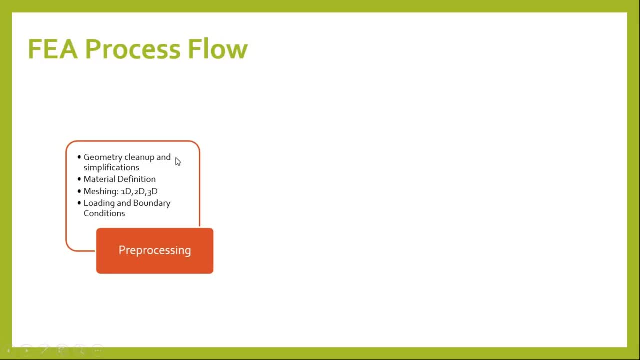 complex kind of feature like chamfers, fillets or any unwanted hard edges. you can clean up that or remove. Then you can define a respective material details and then you model. if you create a FEA model based on 1D, 2D and 3D limits and then put your loading and 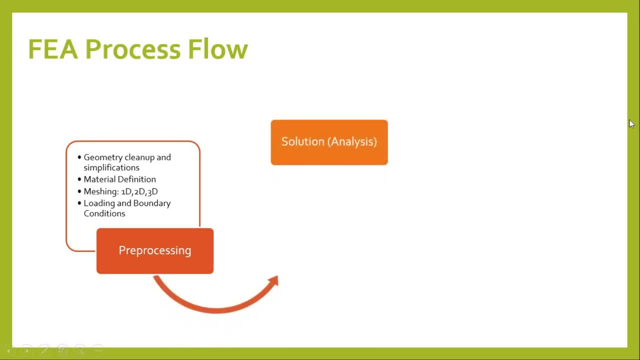 boundary condition. So this is nothing but your pre-processing. Once pre-processing done, then next phase will come, your solution, or called as a analysis. So here, like the major things like what are the types of analysis, what kind of software we need then, is there? 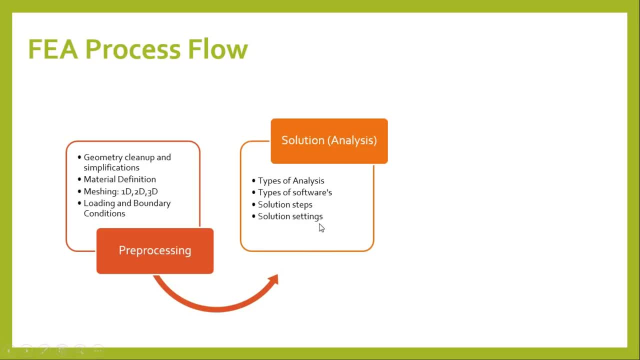 any additional steps are there and then solution set. So these steps are come under solution. So once the solution is done, the next step will come right. your pre-processing. So pre-processing is nothing but your result extractions. So what is pre-processing? So pre-processing is nothing but your result extractions. So 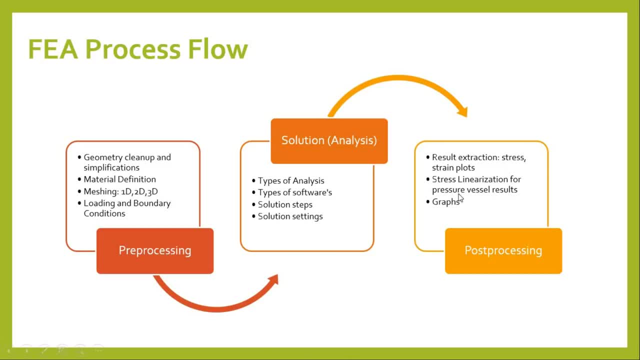 here like stress strain plots, stress linearization for pressure vessels and graphs if you want. So this is nothing but your result extraction and validation phase. So complete FEA process is defined by three terms: pre-processing- where the geometry clean up, and your FEA model. 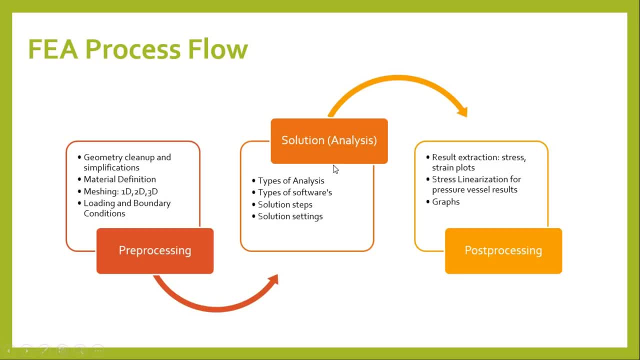 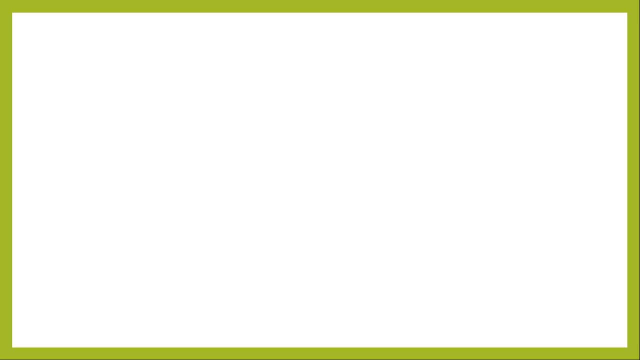 creation is done, Then solution, where we will fire the run and then next is your post-processing, where we extract the results and validate with the design. So these are the major steps to do with any kind of FEA problem. Now we will move towards, as we saw, that FEA process flow. Then, as we saw that there are, 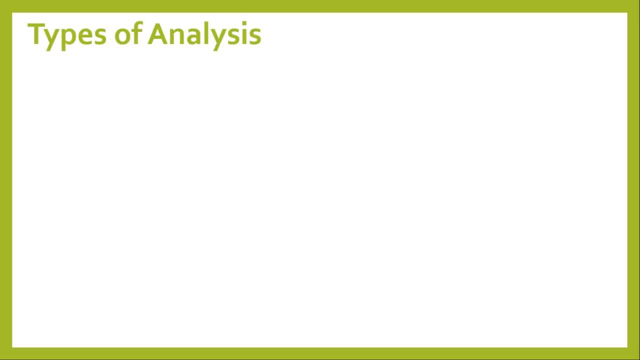 second term like solutions. so here that we should know about what kind of analysis are there, because FEA belongs to the different analysis terms. So what that analysis? So we will see in this slide. So first the very important, All right, 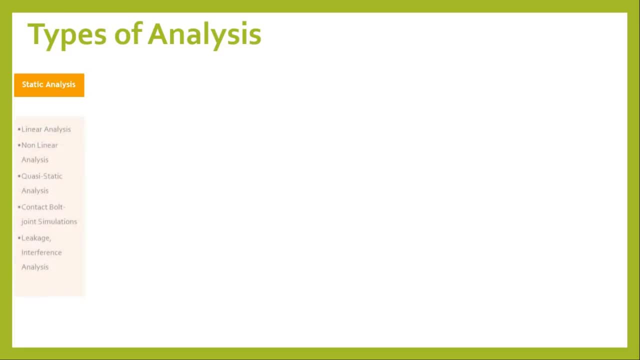 nowadays, most of the industries are doing static analysis. so static analysis is nothing but your simple linear analysis, right? so here, like static loads will come, like pressure, dead weight forces, all these things will come over here. so under this, like linear, non-linear. non-linear is like based on. 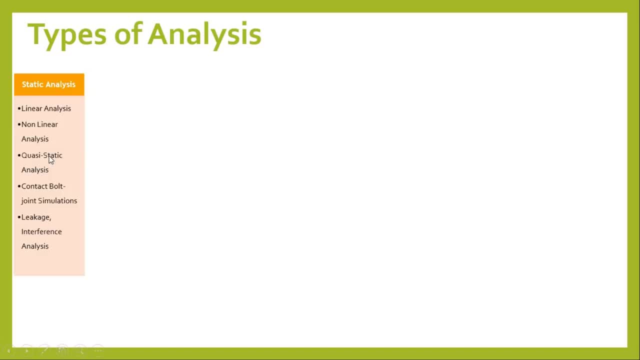 your context: non-linearity, geometry, non-linearity, then it causes static when there is a small times of four sauce layer, then contact bolt joint simulations, then leakage analysis, so these analysis will come under the static analysis phases. then your dynamic analysis come, dynamic vibration analysis come. so you're like: 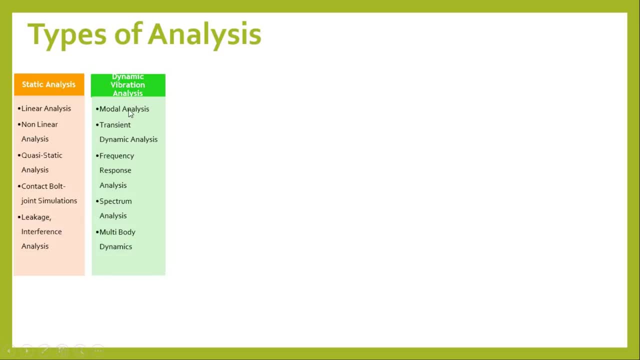 first we uh and basic analysis, your model analysis, from where we will get the number of mode shapes and your natural frequency of the product. then next yours, transition, uh, dynamic analysis here, like loads are there, then frequency response, then spectrum analysis- this is also called response spectrum, like seismic analysis- and then your multi-body. 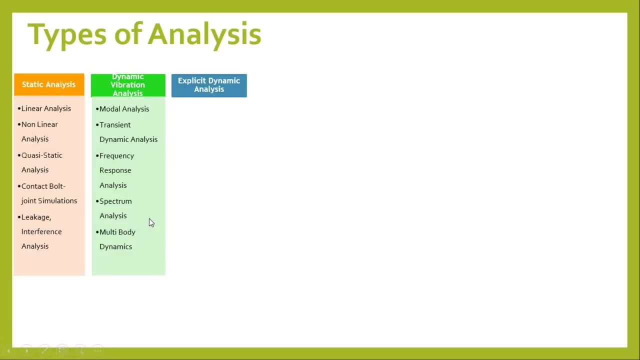 dynamics. so these terms aren't comes under the dynamic energy. the next: we like explicit dynamics analysis. so explicit dynamic is nothing but when there is a small impact is there drop trace can crush projectile impact. car crash analysis: all of us know that car crash analysis impact also. I think most 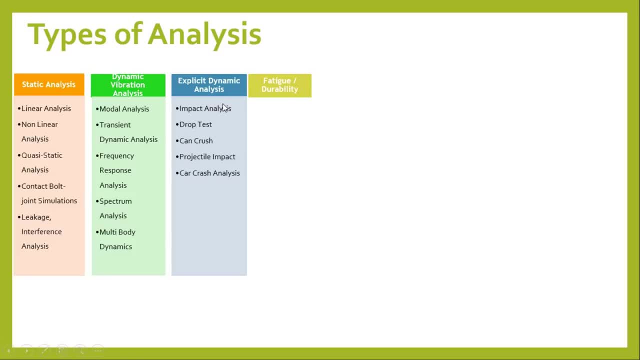 of the people knows, like mobile drop from certain height. so like that these terms are come under the explicit dynamic analysis. so here, basically, the force is there, sorry the, for whatever the load is applied, but at a very short instance of time, then next term will come your fatigue and durability. so in 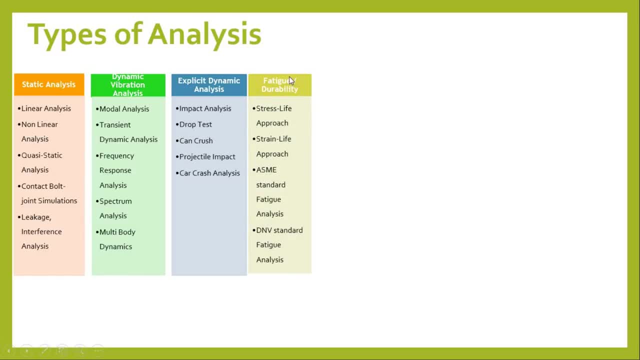 this case, like, as we know, that fatigue is nothing, but you are repetitive load, which will comes for any equipment. consider a case of you are repetitive load, which will comes for any equipment. consider a case of pressure resistance, where it is subjected to different duty cycles. so due to repeat to duty cycles, there some sort of stresses are developed, right so? 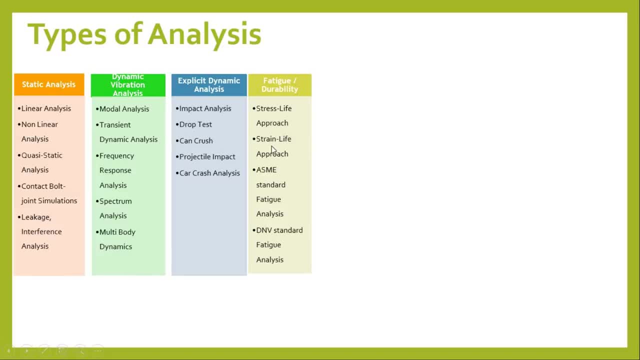 that is nothing but your fatigue stresses. so here, like stress life approach, strain life approach, ASME standard fatigue analysis, DNV standard fatigue analysis, so like that this analysis will come. then thermal analysis. like all of us know that when there is a temperature, loads are there. so the 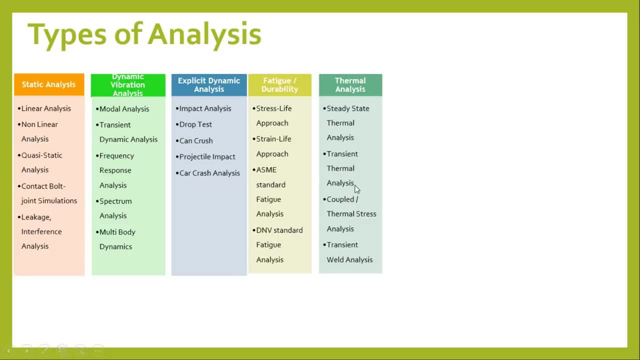 steady-state transient with respect to time. if thermal is profile is varying, then coupled thermal stress analysis transient. well, also, is there like while doing welding there's a high stress stresses were going to develop due to contraction and expansions. so these are conduct the thermal asses. then next term will come like optimization, right this. 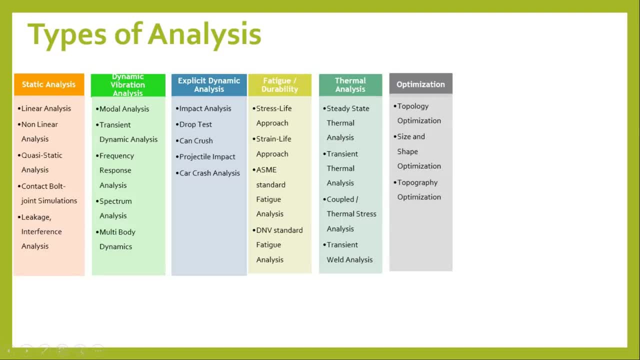 is also most of important terms which is come nowadays used by most of the industries. so the topology optimization, size and shape optimization, topography, after addition, so all these terms are come under optimization. basically, topology means if you apply some sort of force on a cube, based on that force, 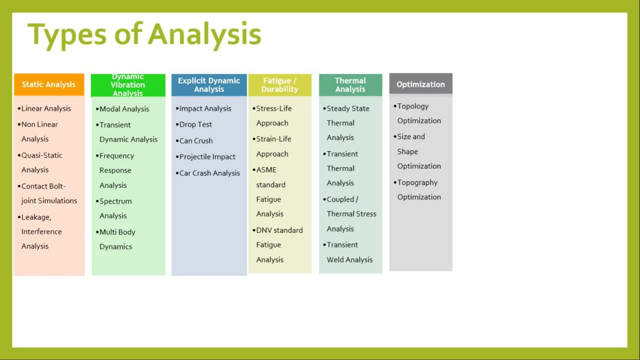 you will get some sort of profile where we need to add a material or where we need to remove the material. so if you remove some material, then based on that for load path profile we can create a geometry from that cube. so this is come under topology and size and shape, like if we have 10 mm of thickness and if you 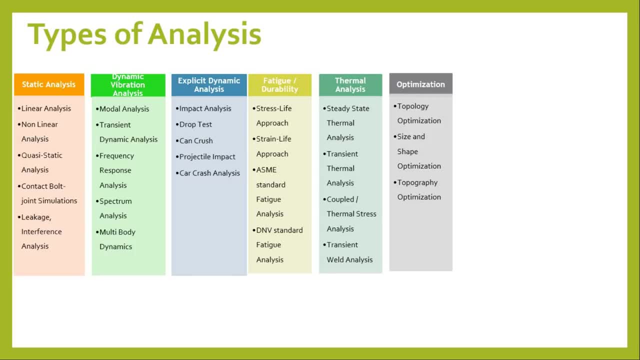 want to reduce, and then that can also be done for respect to loading and respect to thickness, so you can vary the thicknesses based on your loading right. and then your topography means there is some sort of beads or speed patterns you need to add, so like that this software 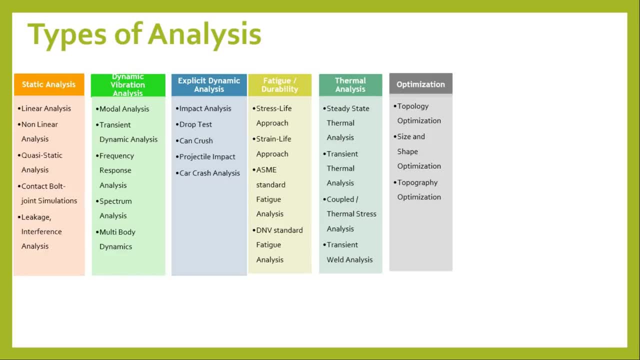 will tell us whether you need to add a patterns or kind of thing so that steepness will increase, so that all these things will come under that optimization. then there are, like high-end analysis- we know that like more analysis, multi physics analysis are also there, like fluid structure. 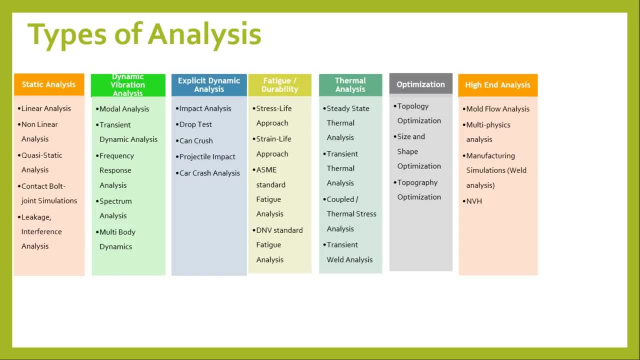 interactions are there when any CFD based analysis, CFD plus FE analysis will come into picture. that is nothing but your high-end analysis. so multi physics like. take an example of any pressure vessel. so pressure vessels, suppose the transport loading condition when it is loaded on the vehicle. what will happen if suppose liquids are there? 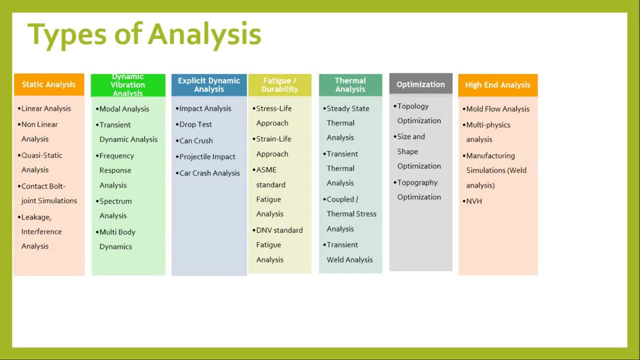 due to fluid sloshing there will be some sort of vibration will going to come and due to these vibrations or sloshing loads, their stresses are developed. so that is come under fluid structure interactions. so this is the analysis that we are going to do in the next class. 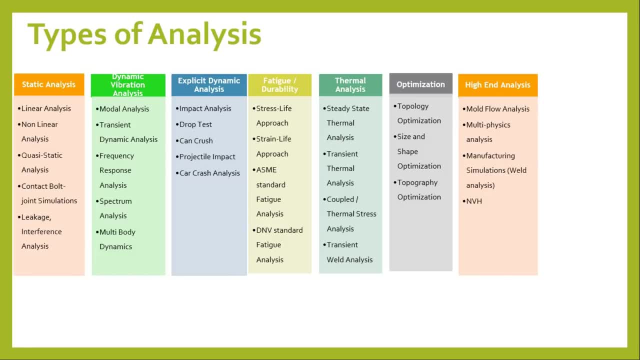 right. so multi physics are there and now NVH is also this: noise, vibration and higher, and is the next last term will like CFD, that is, computational fluid dynamics. so here, like if you wanted to know that, pressure drop ratio, flow characteristics, cavitation study and thermal transient flow analysis, laminar. 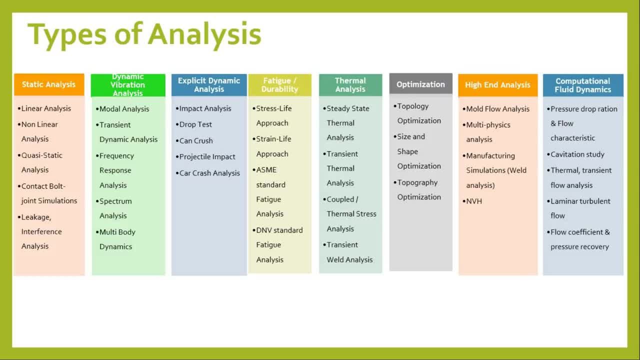 turbulent flow coefficient, pressure recovery. so all this come and does the computational fluid analysis. so this slide is nothing but a brief you. what are the kinds of analysis are available in the next class available and in the commercial software. so all the analysis will come under this. 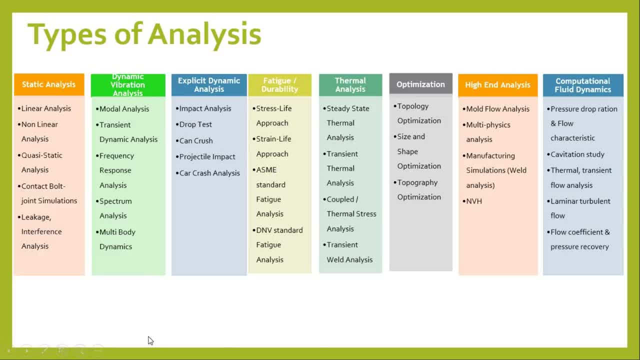 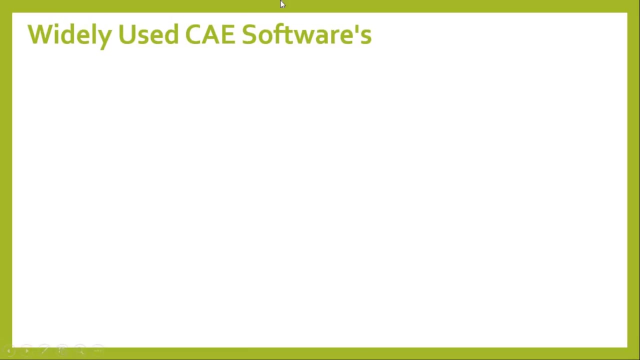 so eight tabs, so so right. so if you get a chance to go through each and every in depth, then you will come to know what exactly these are. okay, when you try to solve this, then you will get the more idea on this. then next, we know that there are different analysis, are there, but for this? 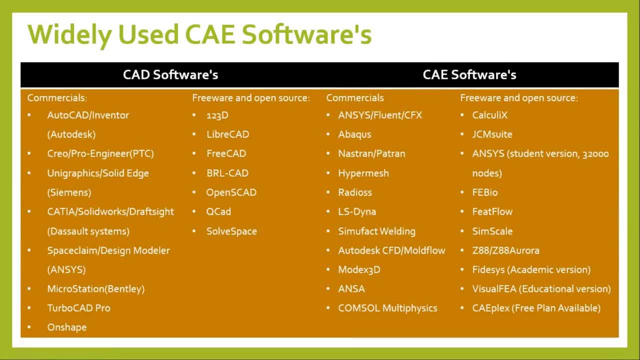 distribution analysis. there are also different softwares are available in the market, like when we talk about CAD software, so they are like commercial CAD softwares are like: mostly use AutoCAD, inventor, Autodex, the product of Autodex, that Creo. product of PTC uni graphics. product of Siemens: Katia solid. 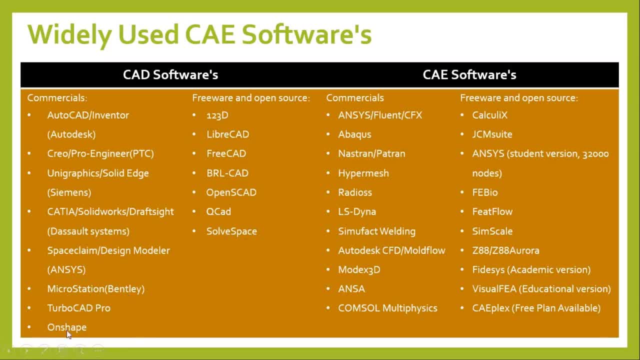 work space claim, micro station Bentley on shape turbo CAD Pro. so these are the commercial softwares and there are also free softwares or you can say open source are available so you can get. if you don't have a license for this, then you can refer this license like one, two, three CAD in Libro, CAD, free CAD, BRL CAD. 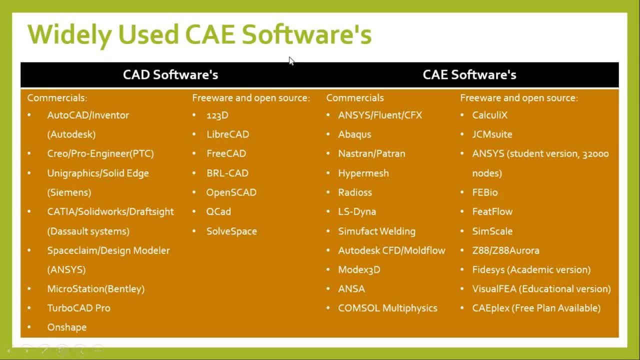 opens CAD, QCAD and solid space. so these are the free softwares available. you can download that from easily. Google then see softwares as we know that and sees fluency, Apex, abacus, Nast and Pratt and hyper mesh ready use LS, Dinah Simu. 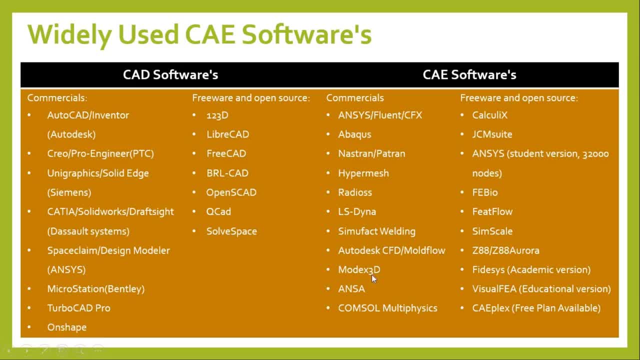 fact, welding. this is for welding- Autodex, CFD, mold flow, mode X, 3d, ansa, Cosmo and multi physics. so ansa is also like pre-processing software and also will come like hyper mesh kind of thing. these are pre-processing, so and these 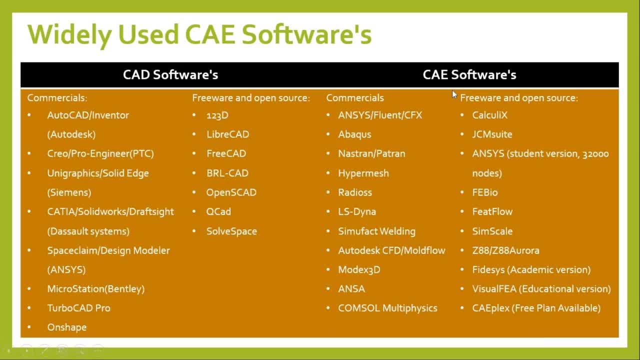 are like solvers, abacus and see is passed on pattern and they're also like free or open source software available. see softwares when we talk about Cal, Calculus, GCM suits and see students versus not all over for like 32,000 nodes. so this is basically biomedical engineering. then if you feed flow for 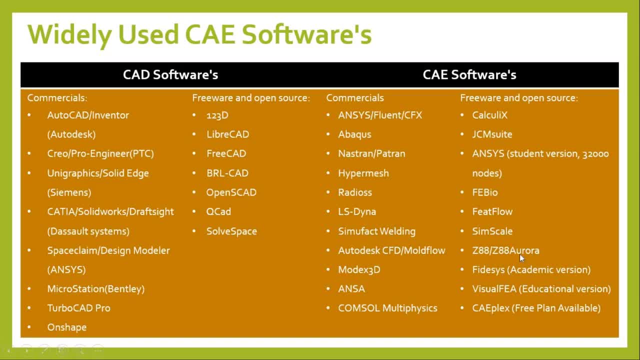 CFD same scale, then your jet double it. the aura, then fit say this is also like academic version. if student want to refer you, they can refer this visual FEA educational version and see plex also free plan available for this. okay, so these are like commercial as well as free softwares available or widely used. 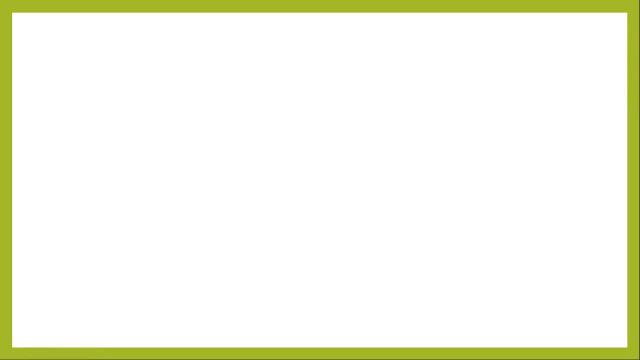 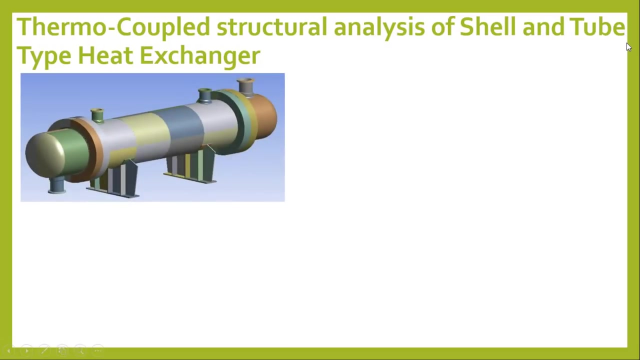 in the industries. then we will talk about different examples or we'll go through the some of the examples of this FEA. okay, so first example is like thermocouple: structural analysis of shell and tube type heat exchanger. so we'll go through this. this is what your heat exchanger that is called shell and tube type heat. 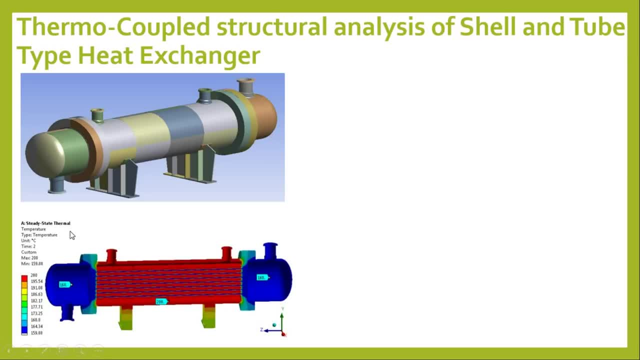 exchanger and for you can see that once we will apply a temperature change temperature from shell side and tube side, you will get this kind of profile. so your temperature, this is the body temperature plot here, like, temperature is varying from 200 degrees centigrade to 159 degrees centigrade, so 200 will be. 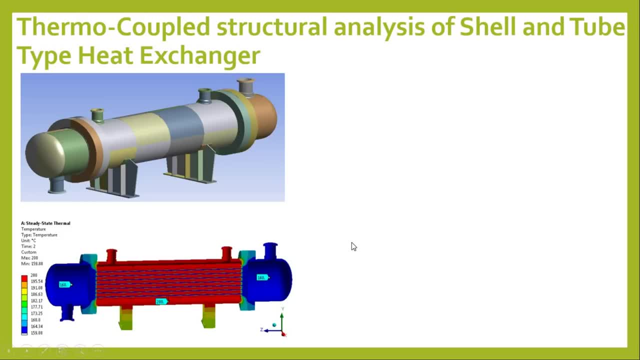 on the shell side and here like tube side. so all of us known that. what is shell side and tube side? let me explain that. when the fluid will enters into this, like from this, and it will go to pass through this area to side area and also inside the tubes, that is called the tube side and shell. 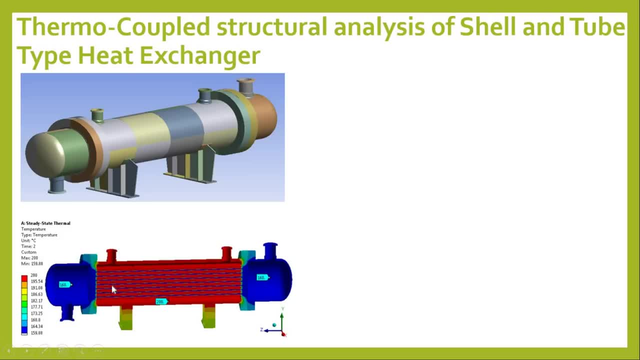 sys is nothing but when the cold fluid will flow through this and it will pass through out of the tubes and it will move out from this. that is called the shell site area. so like that, there is a. two different foods are there, which is having a two. 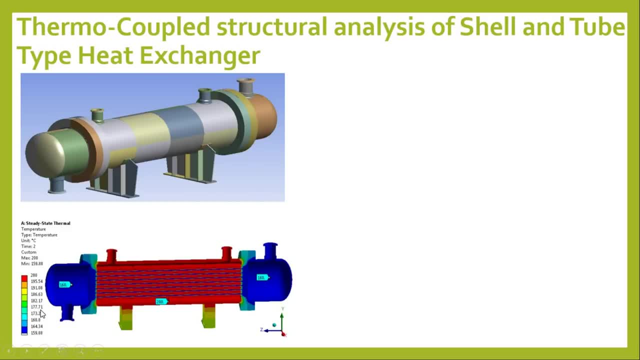 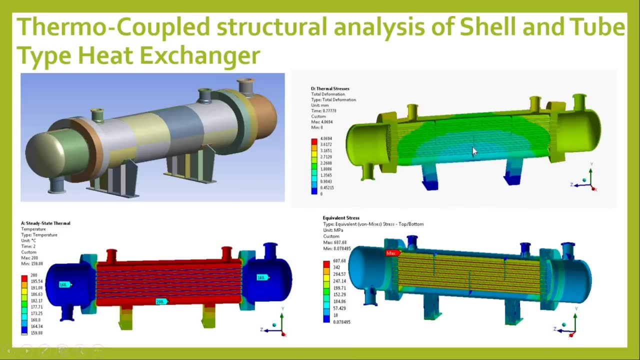 different temperatures so far that we need to do this thermal simulation right and this is what your equal instance is for that and you can see how it is viewing for that respect to temperature load. here it is fixed and along this fixing it is try to expanding due to the temperature difference and these are the stresses you will find over here. 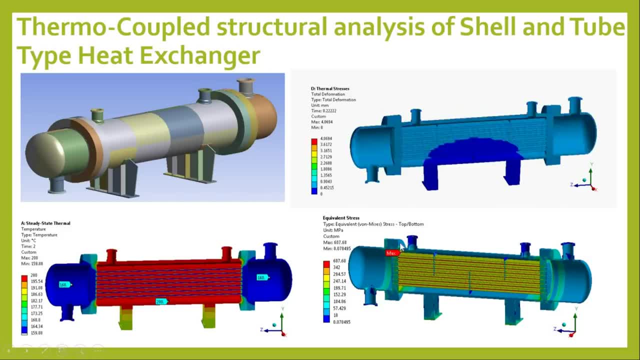 like maximum stress are will going to find your here because there will be the more temperature gradient at these junctions. that is called the tube sheets. okay, so this is one of the example of thermocouple structural analysis. once your thermal loads are applied, there also some additional. 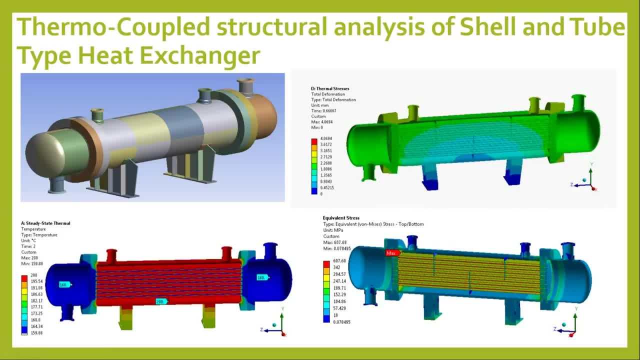 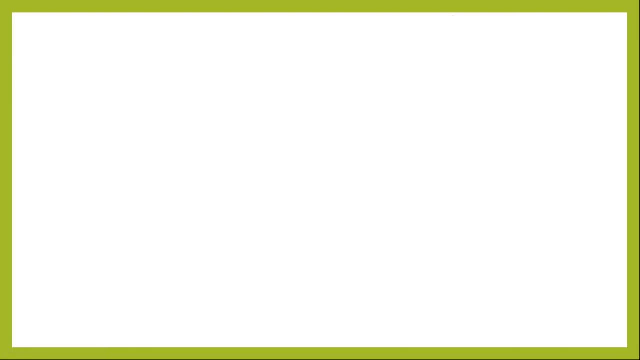 pressures are there, like, similarly, shield and tube side pressure. so that's why it is called thermocouple structural analysis. so first you need to fall the thermo analysis, then you need to couple that with the structural analysis. in structural you can apply a pressure loads, okay. the next example we will discuss about the hotbox analysis of naphtha stripper vessel. this is also. 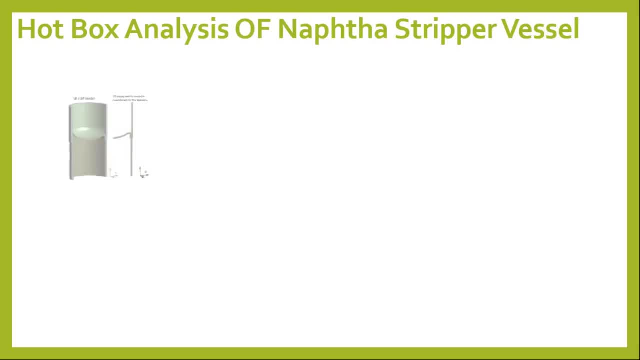 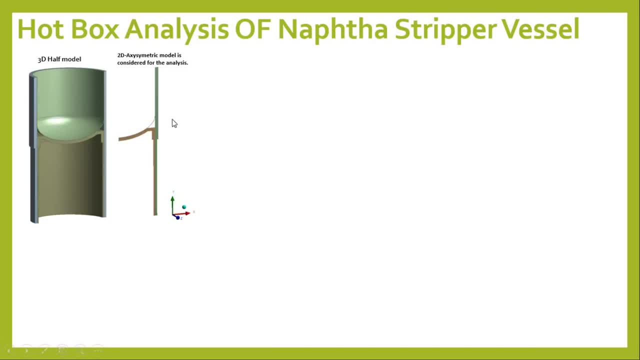 so here, like, uh, we will do the axis symmetric like 2d analysis. first we saw the 2d 3d, now we will going to see the 2d analysis for that. but this model is axis symmetry along the center axis, so we first we can extract this 2d shape and then we can do the simulation so it will save over. 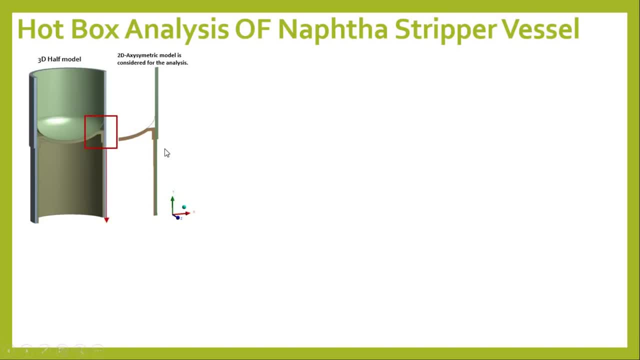 time as well, as we will get the less effort to do the machine right. so you can see, this is nothing, but your shell in between skirt is there. this is outer insulation and this is inner insulations. so this portion is nothing, but you are a hogsball. the purpose of this hot box is nothing, but because 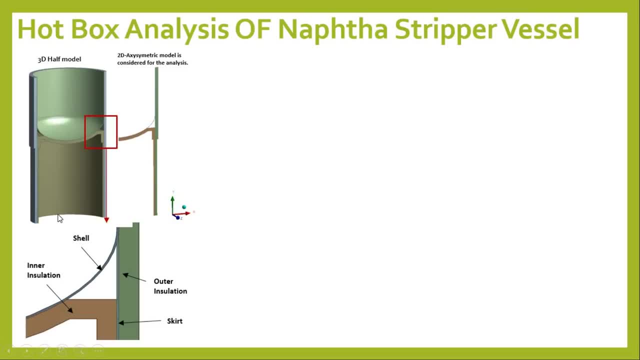 this shell are subjected at a very high temperature, so this high temperature should be pass out to this. so due to this radiation, or you can say due to this hot box, it will going to pass to this steepers right. so that's why you will get the very less stresses at the junctions. so that's. 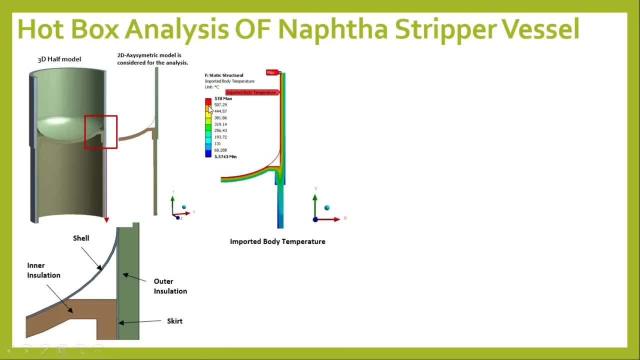 why this hot box are provided. now you can see the imported body temperature. once you will do, do this thermal simulation, you will get the temperature profile like this you can see right, and these are: once the thermal is done, then you can do this static analysis where you will going. 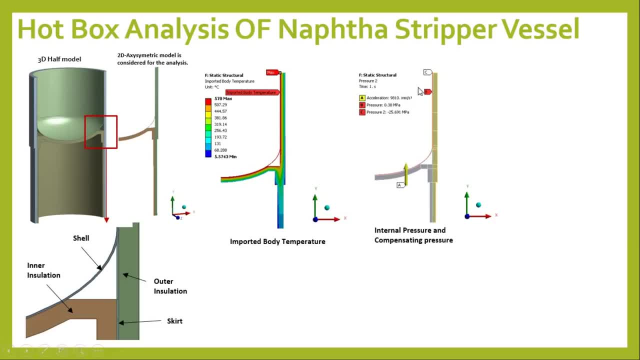 to apply the G loads, your pressure loads, internal pressure on this facial right and that combination compensating pressure at the opening, because we haven't considered complete portion. so that's why we need to apply this and this is what you are due to this pressure loading. you can see the 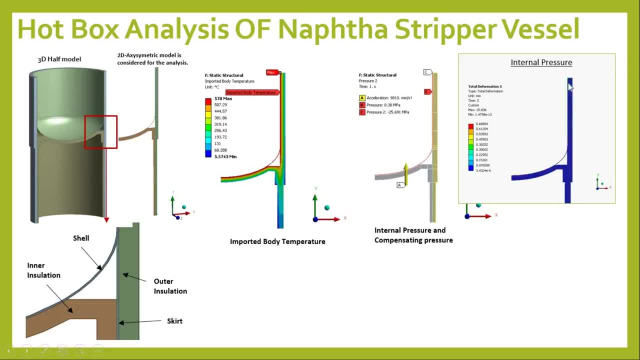 deformation, how it is deforming kind of thing. so it is trying to moving out or you can, radially expanding along the this fixed location. okay, so here and the due to temperature, as we can fix from this, and due to temperature it will try to expand and due to pressure it will try to. 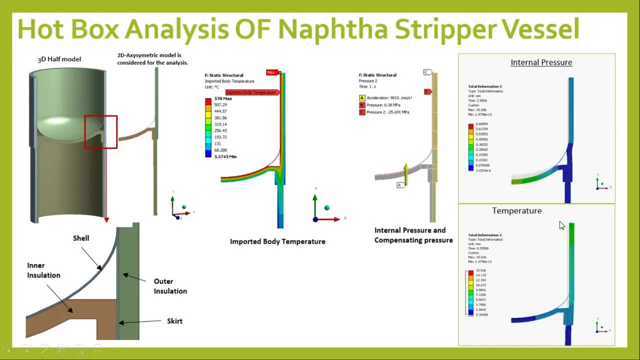 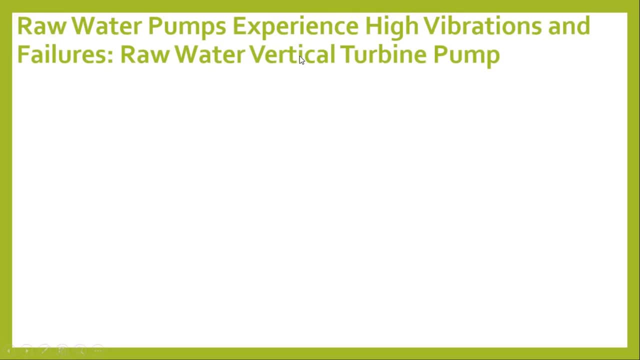 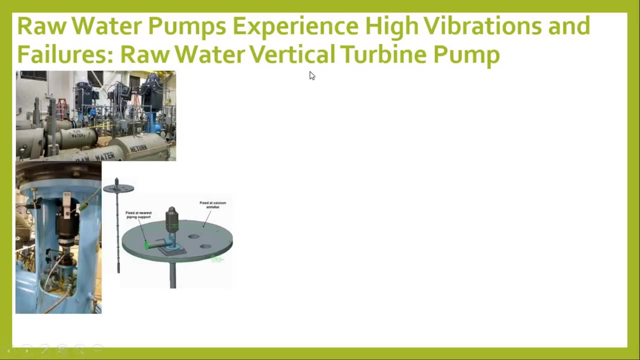 move out right. so like that, once you will apply the loads you will come to know that this kind of profiles okay. then the next problem. we will see one of the example of raw water pump experience: high vibrations and a failure. so raw water vertical turbine pump that is called route. 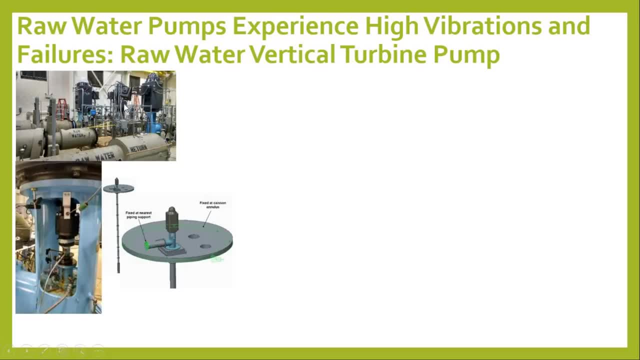 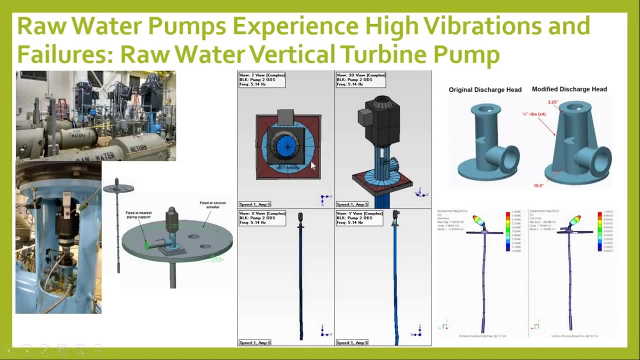 what if you can see? this is nothing but your the actual configuration and this is what your router turbine pump. okay, so you can see. first I will put all the plots so that you can able to see how it is deforming, how it is vibrating. if you see one of the example of this, first with this: 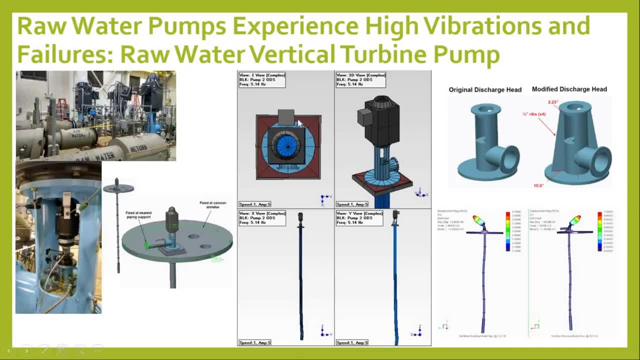 position they might getting the. you can see the deforming, the natural frequency and your mode shape will be like this, so you can see the animation that is right here. also, you can able to see the submerged portion of this which is vibrating and having the frequency of five one one four. so these plots belongs to them. respect to more shows, which is: 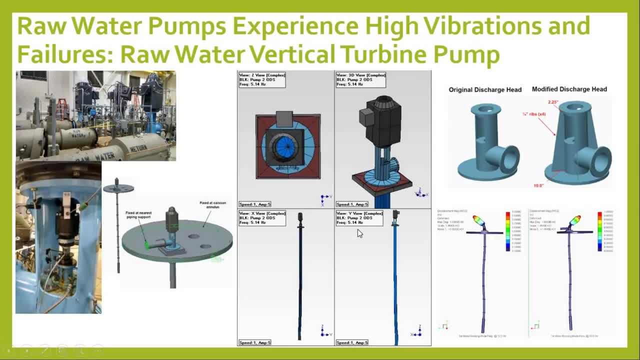 I am frequency point five. point one four, right, so this might be exciting with their operating frequency. so once your natural frequency will excitedly or not, excitation frequency, then your resonance will going to happen. so for that, if you say that your natural frequency will excite to be, 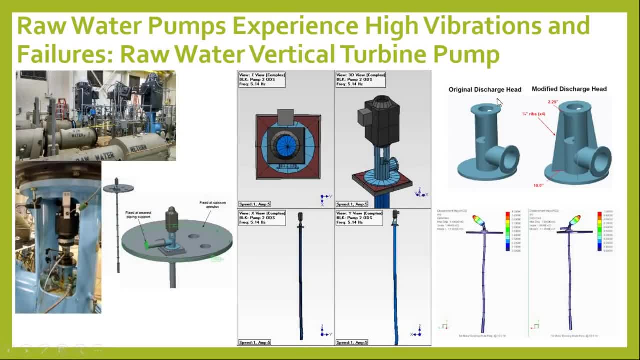 your enough excitation frequency then your resonance will going to happen. so for that, if you see, this model belongs to this category: original discharge head. so what they have put it. they have added this rips- you can see this rips to get the additional steepness at this pump locations. so 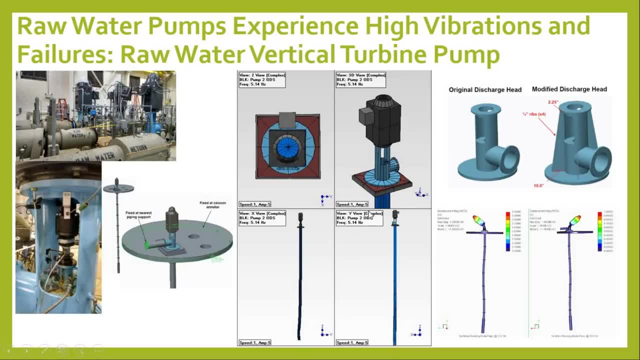 once that is done, then they will get the some sort of shifting from this frequency right. so you can see this, the virtual displacement plots, so like that. when you come across these some of the vibration simulation problem problems wins. the problem belongs to the coincident with natural frequency, so in that case you need to put some sort of additional rips or you can. 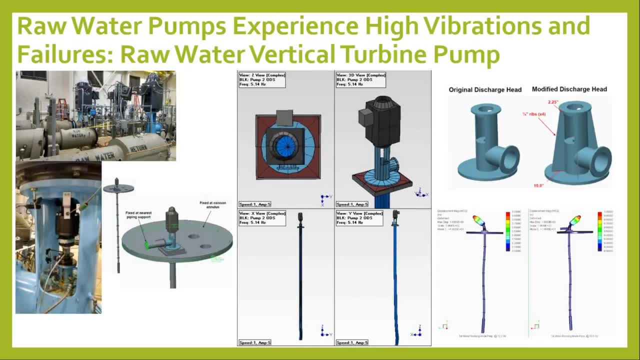 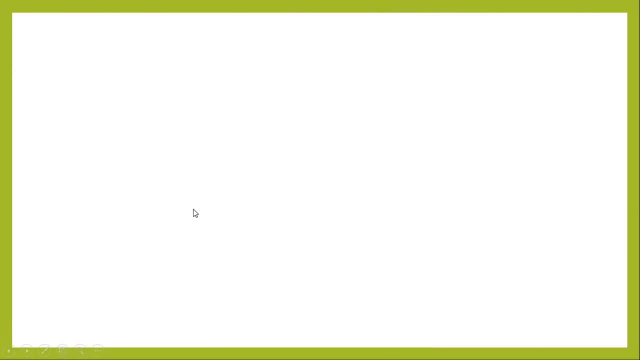 strengthen that model so that we can shift that frequency from the net natural frequency right, so we will reduce the chances of the resonance in that cases. so this one of the case study. I had a refer from this reference. you can go through this reference for more detail. okay, now next case study. 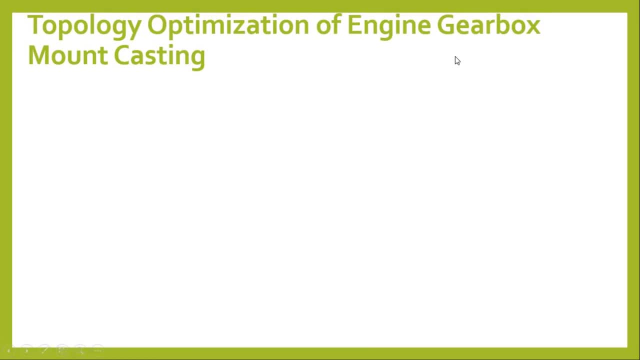 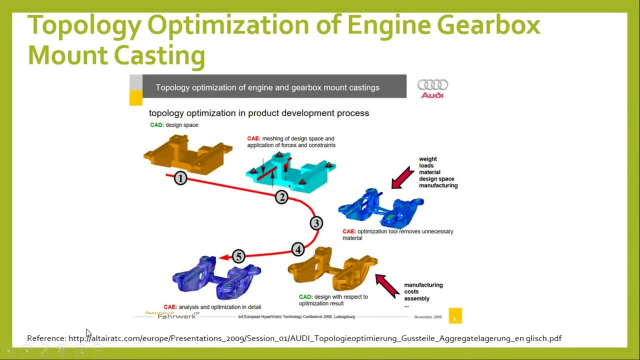 this is also very interesting, like topology optimization of engine gearbox mount casting. so here, if you see, this is the topology optimization of engine gearbox mount casting. so here, if you see, these are the one of the example from Audi, so they used to do this topology optimization, if you see. 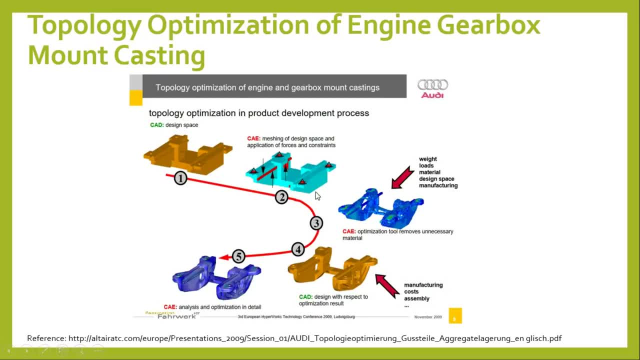 consider the design phase. this is what the initial model, and then you need to apply a load and fix this. based on that load, you will get some sort of profile. now you can see the weight loads, material, design, space, manufacturing- here you can put the manufacturing as well as design constraints. so 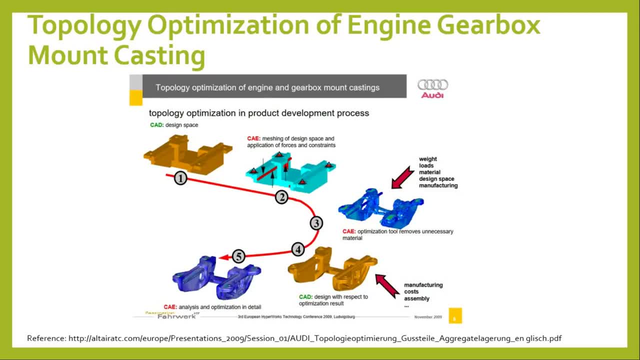 design constraint is nothing but you are fixing location. manufacturing constraints means if you want to some under some of the manage, if you want to keep for a manufacturing point of view, to get the standpoint of you, so you can define that as in under the manufacturing constraints once you will get the defined profile. 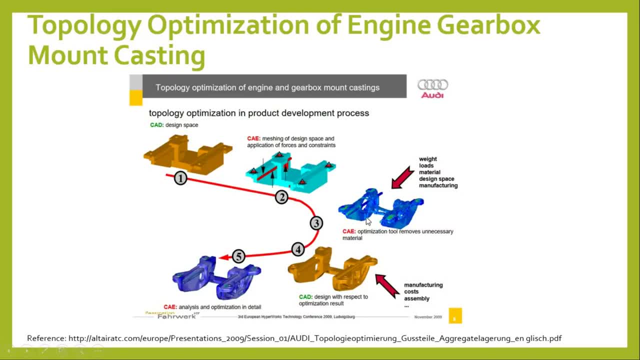 so you can further create a geometry design with respect to the optimization RNite manufacturing cost. so from this you will get this kind of profile and from this prof, based on this profile, you will create this kind of geometry and then you will get the final shape like this and this: 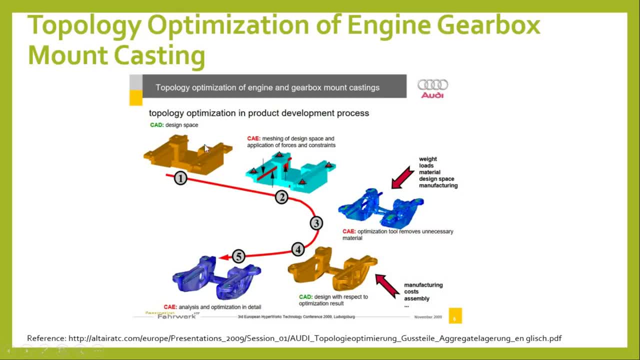 is a design optimization, like the design optim由 الأحاAMA rules. okay, so if you see initial geometry and then let's on geometry, will find a lot of material is reduced, so it will be ultimately saving the cost, right? so like that, this optimization will going to work. so this is also. i have taken some 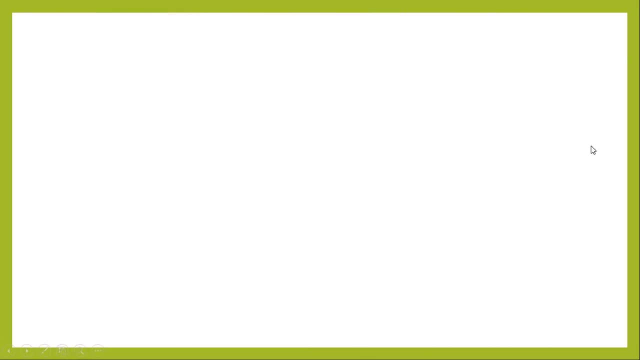 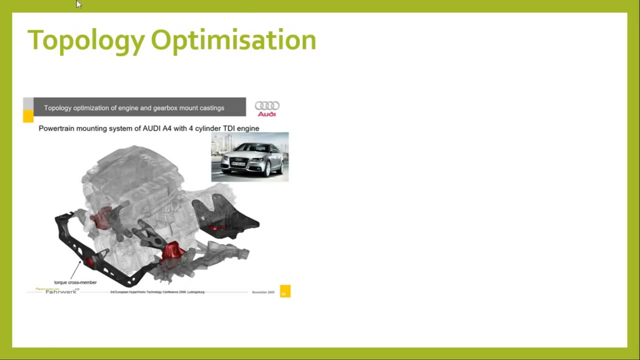 audi reference. okay, so we'll go through the another example, same of topology, because this is very interesting. this is also from the same pdf. i have taken this example. if you see, this is nothing but your torque cross member from the uh powertrain mounting system of audi a4. 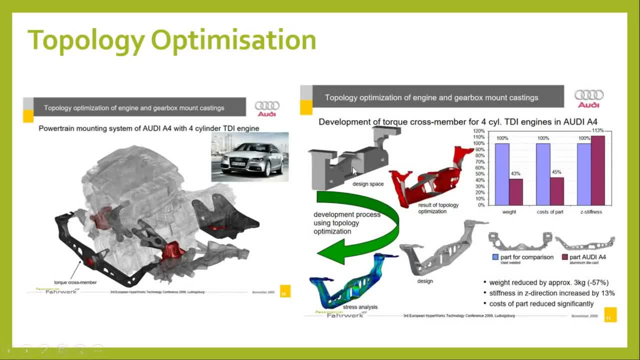 and with four cylinder tdi, right. so here, if you see, this is what your initial design space and based on that we- they- have got this kind of profile. so, based on this profile, they designed this geometry and further did the validation. okay, so you can see the different. 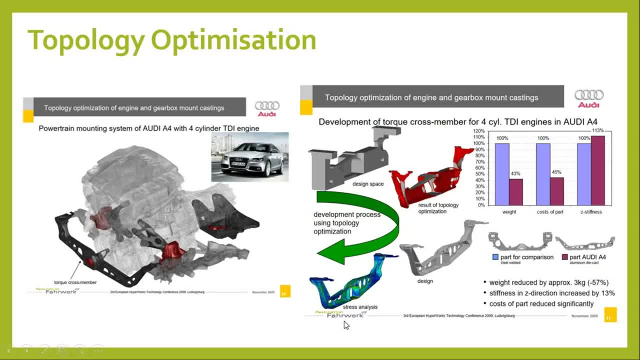 uh processes and based on that you will find that lot of material reduction. so you like weight reduction apply. so if you talk compare, this is nothing but your comparison. your weight: 100 earlier now it is like 43 percent. cost also will reduce like 45 percent and steepness will also increase. so all three 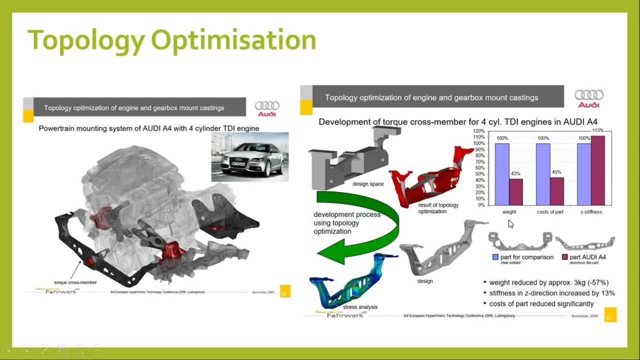 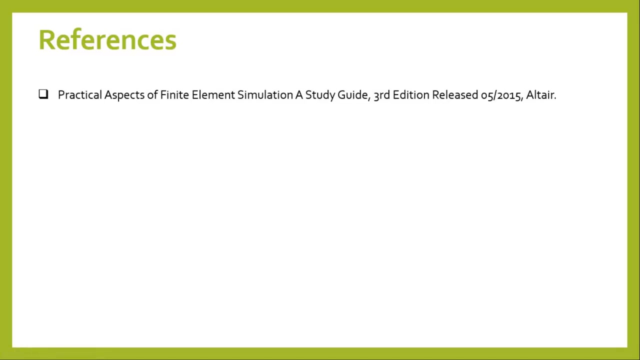 parameters are uh showing the increase in your uh steepnesses and reduction in your weight as well as cost. so, like that uh, when you talk about weight reduction, then you need to think about topology optimization. okay, so these are the references uh from where i have taken uh this complete video, or you can 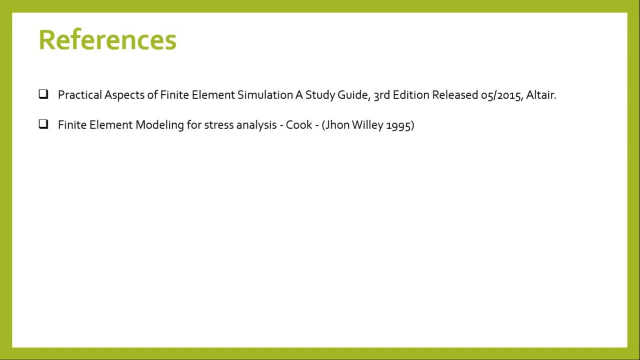 say i had captured this video based on this references. the first will like tactical aspect of fea case study, then finite in the manual stress analysis, then this is what one of the pdf from where i have taken this reference. so these are the major references from where i have. 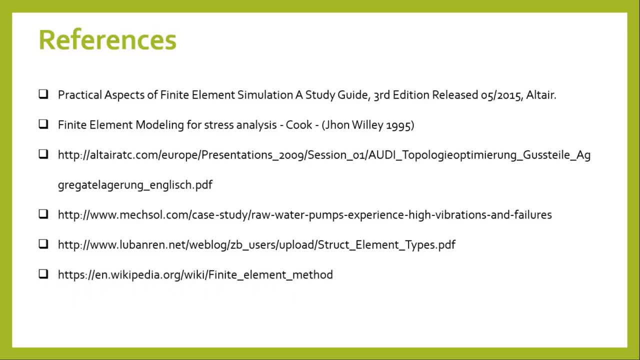 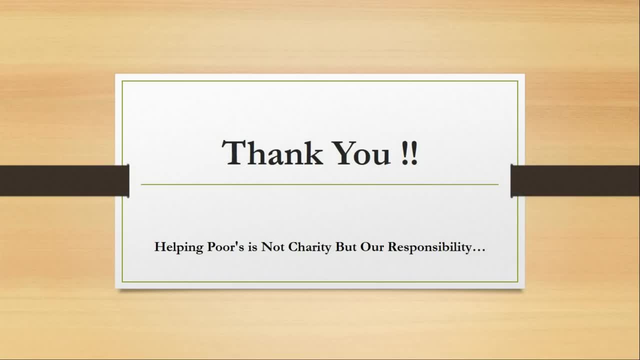 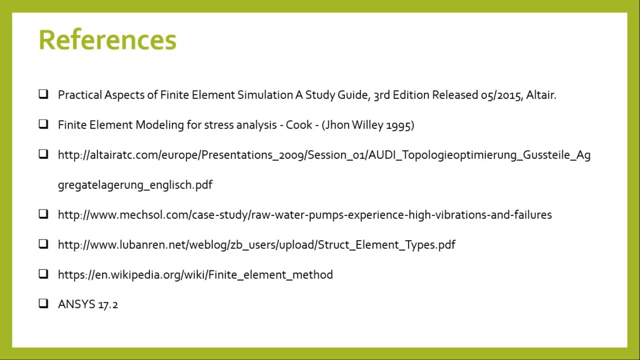 created, uh, this complete video, so hope you guys have liked it, and i had used ansys 17.2 version, so thank you guys, thank you for your time and thank you for keep watching this. okay, hope you will have like. please let me know if you have any questions on this. i'll. uh have to give a try for the next video. if you have any questions on this, i'll uh happy for that. Happy to help you in death.